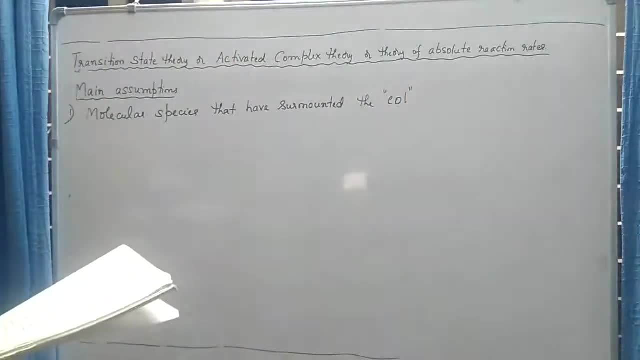 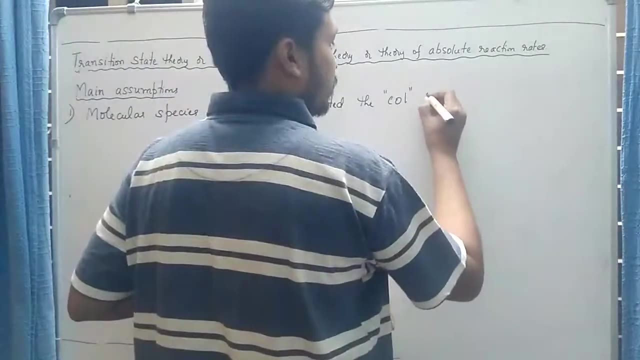 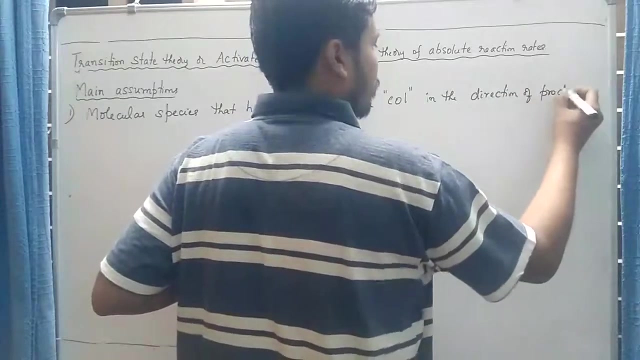 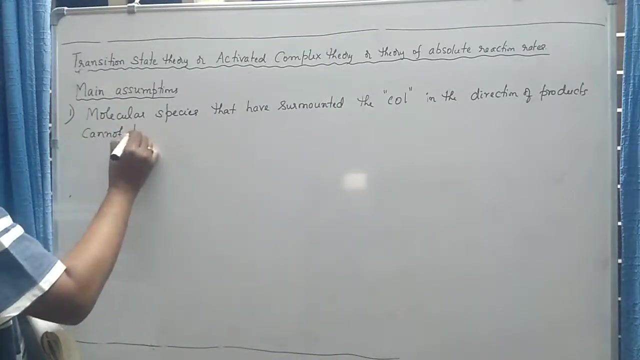 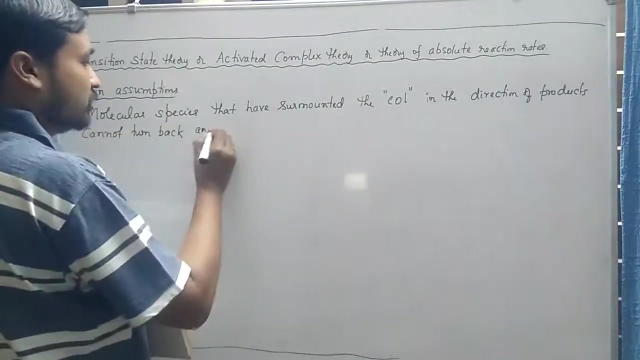 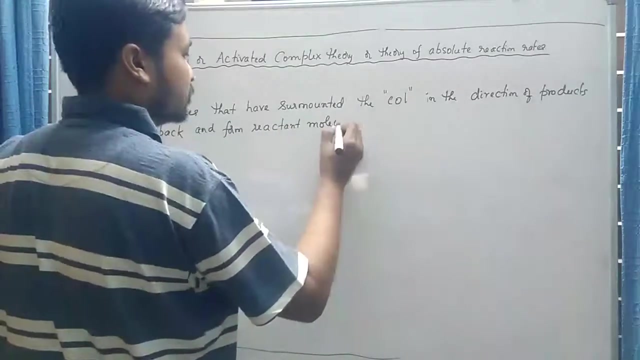 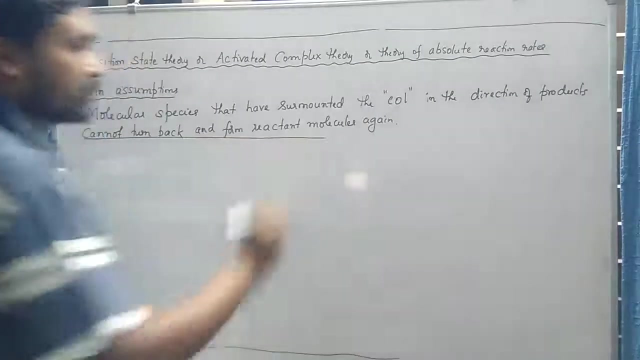 I already told you what is call It is the peak of our potential energy diagram. So molecular systems that has reached or surmounted the call in the direction of products cannot turn back and form reactant molecules again. They cannot turn back and form reactant molecules again. 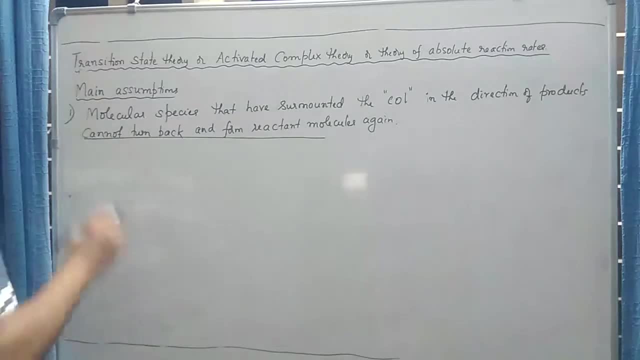 What is the meaning of this assumption? First let me read the assumption again: Molecular species that have surmounted the call. What molecular species I am talking about? It is nothing but the activated complex that are formed at the call. That activated complex, once it is formed. 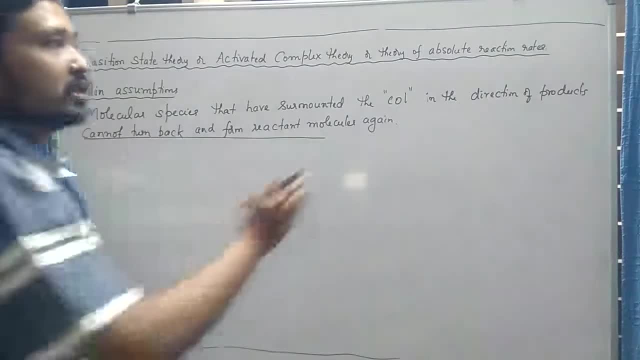 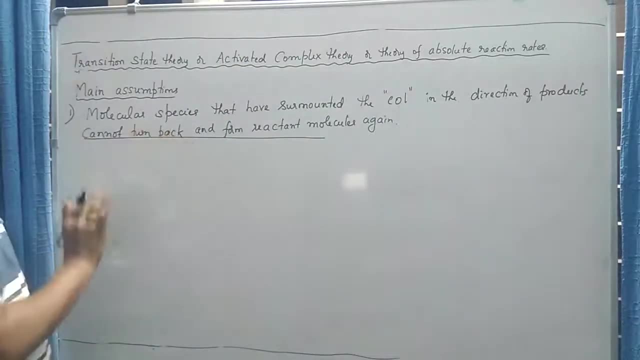 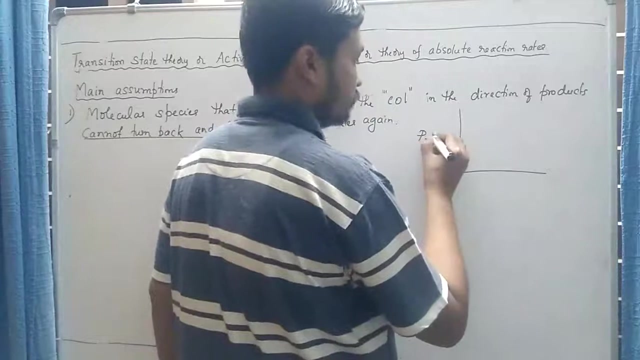 it has no other option other than forming the product. It can move only in the direction of formation of product. It cannot revert back or turn back and form the reactant molecules again. So if I have again draw the potential energy diagram, Potential energy and this is the reaction coordinate: 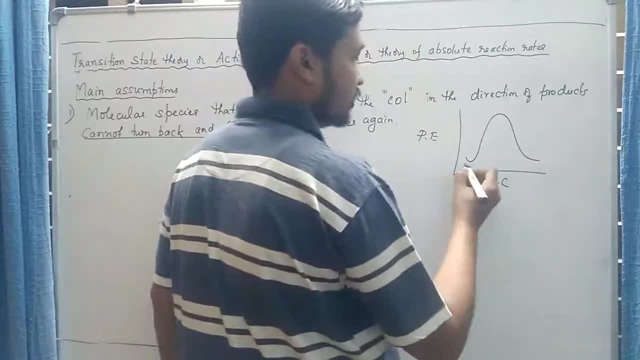 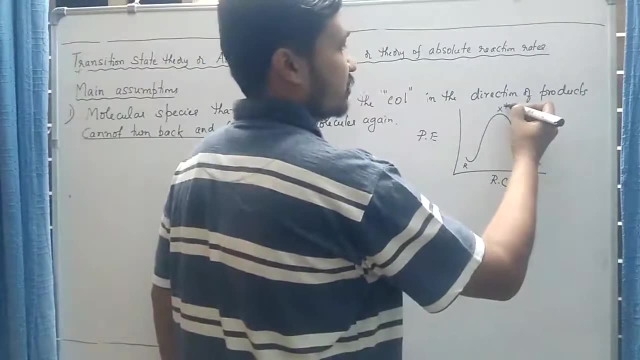 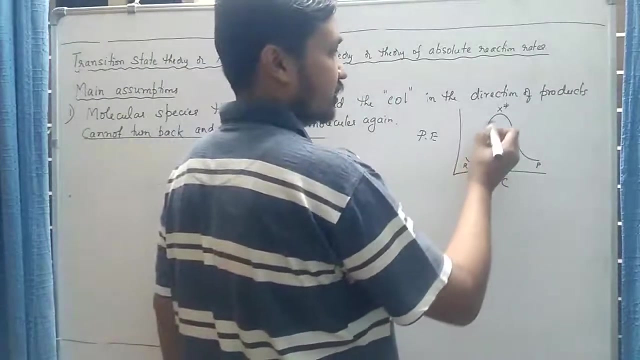 This is how the potential energy diagram looks. So this is the reactants, This is the product side, So this is the activated complex Represented by the symbol X dagger. So when the reactant molecules, after collision, has formed the activated complex, 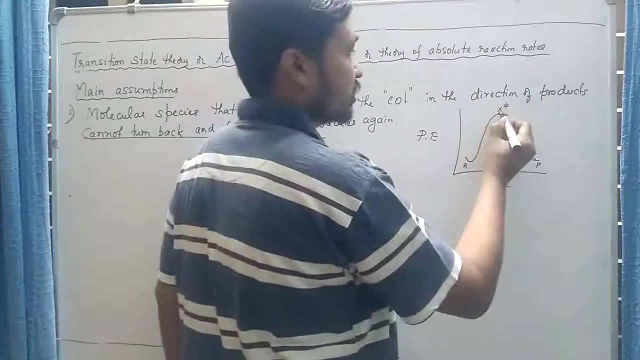 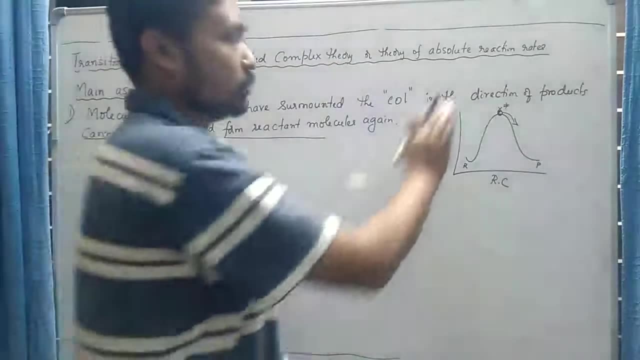 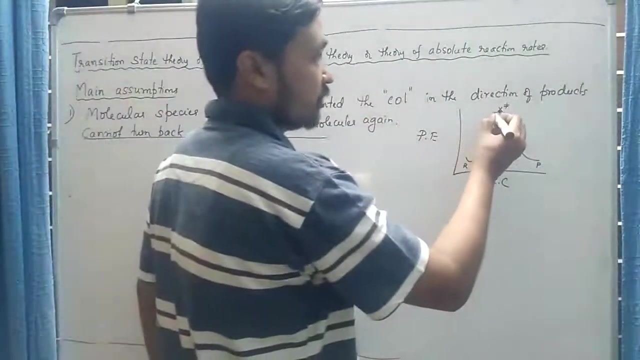 Once this species is formed, Once this species is formed here, This species can only move in the forward direction. It can only move in the forward direction. It can only roll down to form the product. It cannot roll back to form the reactant. 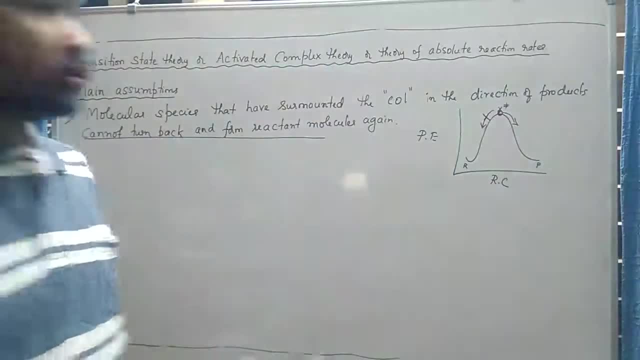 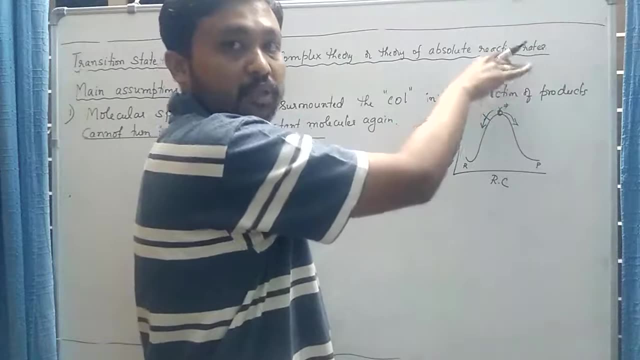 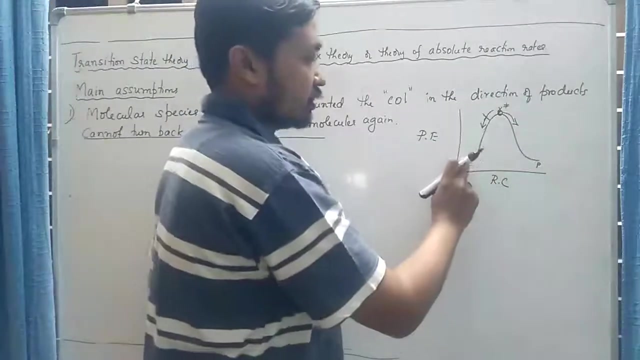 So this is not allowed. So there is only one direction here. The reactant will be converted to activated complex. The activated complex can only move in the forward direction. It cannot form the reactant again. So this process where reactant is forming the activated complex, 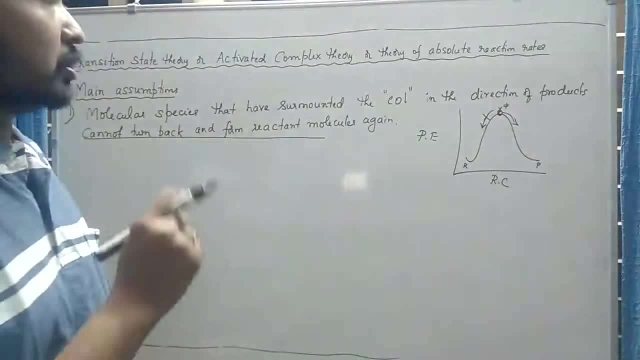 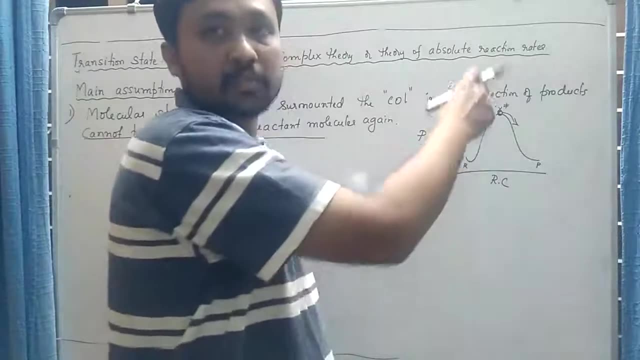 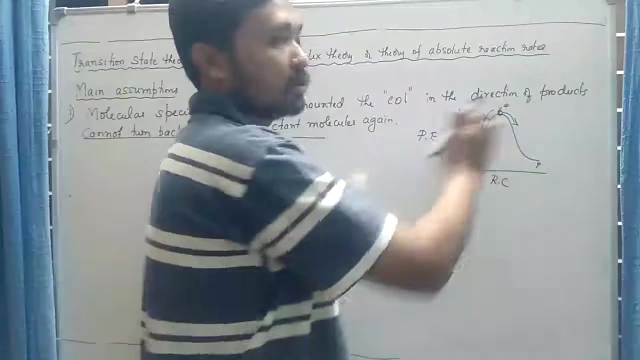 That is a process taking place only in forward direction, So this is not a reversible process. Reactant may form the activated complex, But the activated complex cannot revert back and form the reactant, So this process takes place only in forward direction. 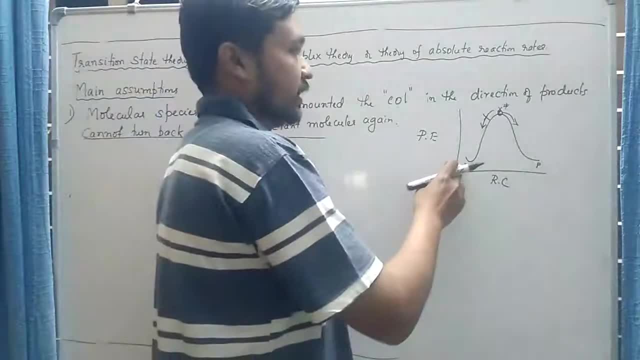 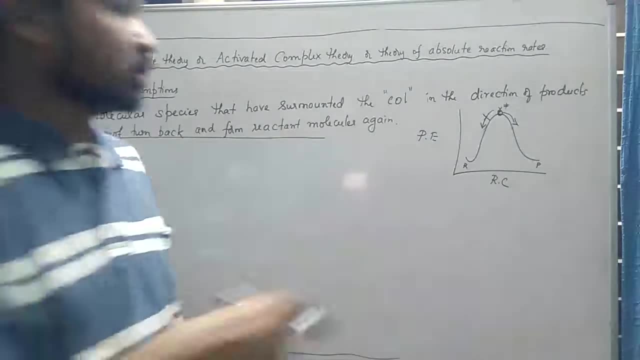 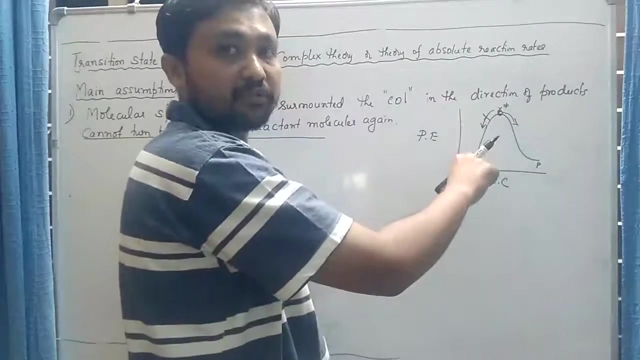 So there is no equilibrium between the reactant and the activated complex. You know that equilibrium is established only if the reaction is reversible. But this process is not reversible. The reactant can form the activated complex, But the activated complex cannot again form the reactant. 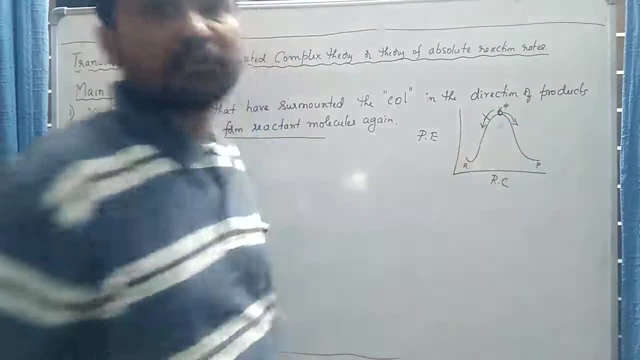 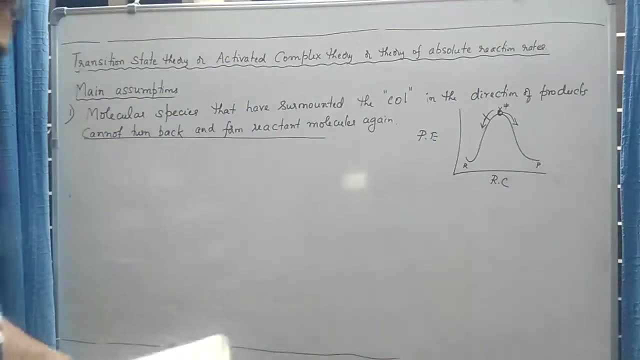 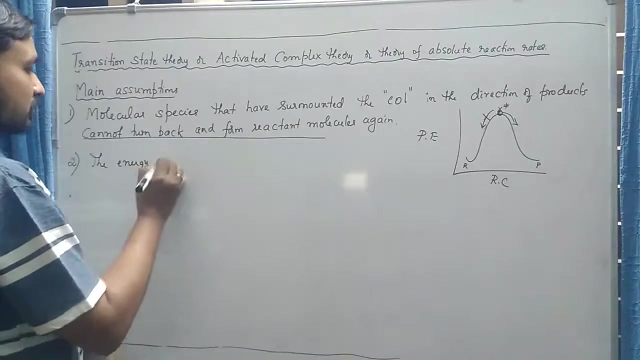 So this process is not reversible in nature And therefore there is no equilibrium established between the reactant and the activated complex. So this is an assumption made by the transition state theory. The second assumption of the transition state theory is The energy distribution. 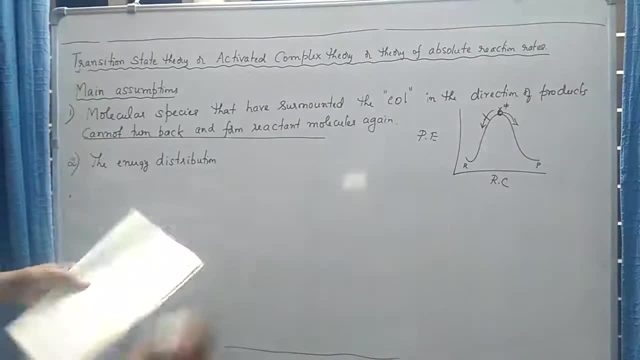 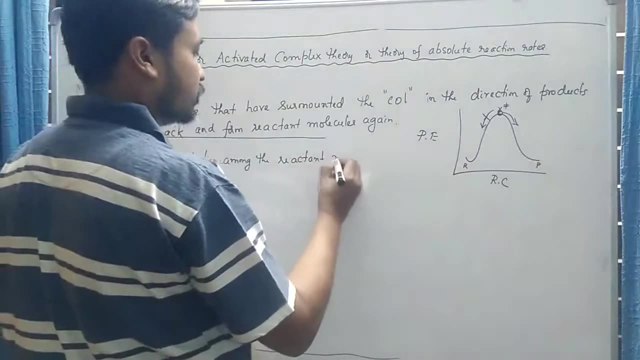 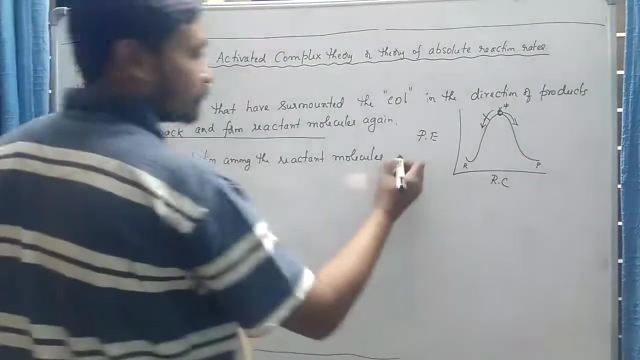 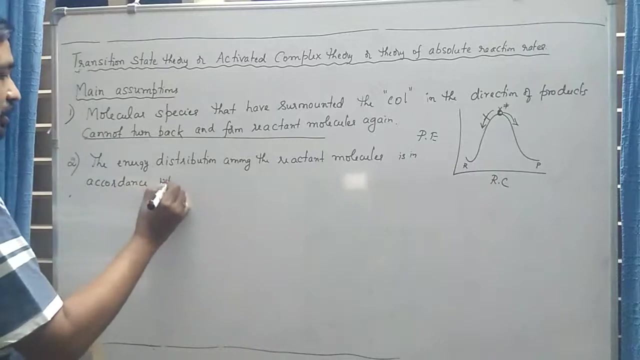 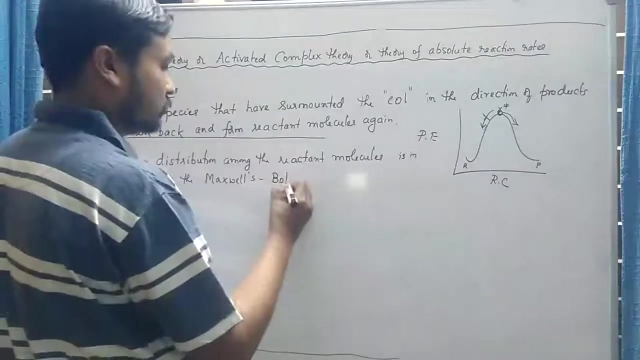 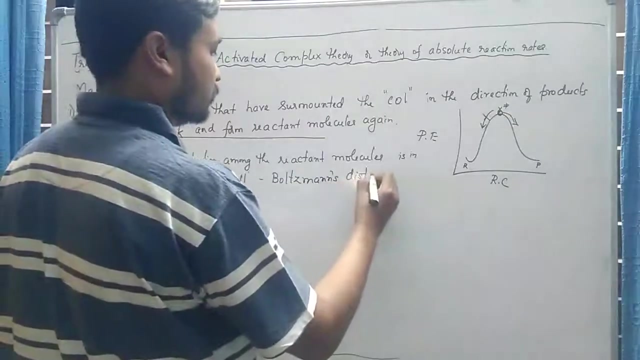 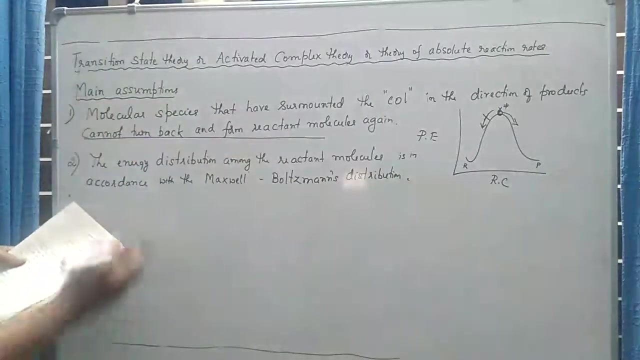 The energy distribution among the reactant molecules. The energy distribution among the reactant molecules is in accordance with the Maxwell's law. Maxwell's law, Maxwell's law 데미역, maxwell goldsman's distribution. further. this is important further. 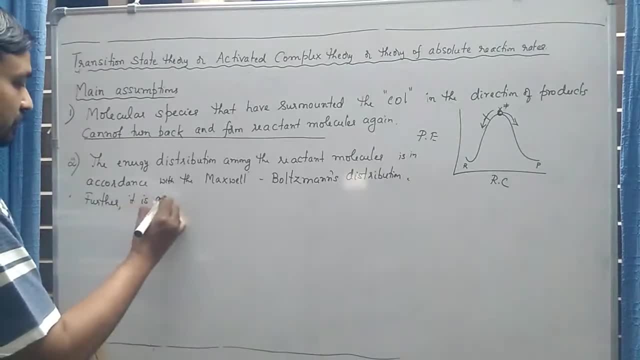 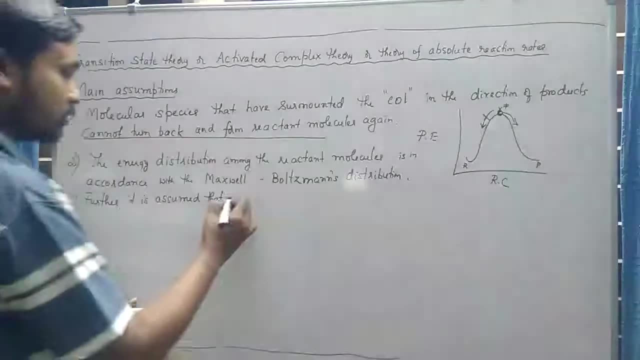 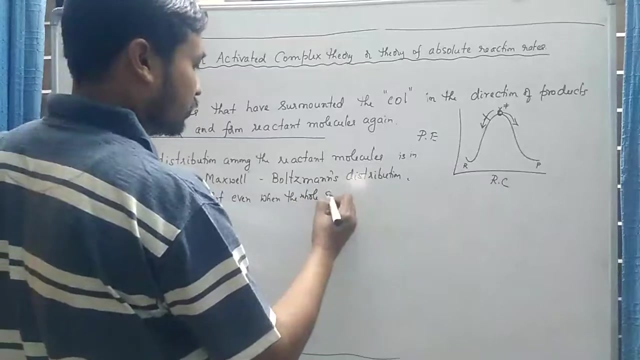 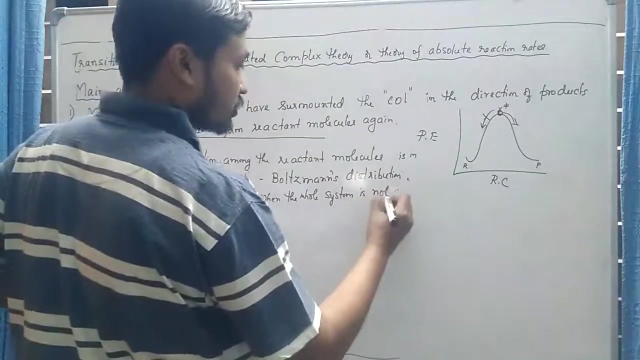 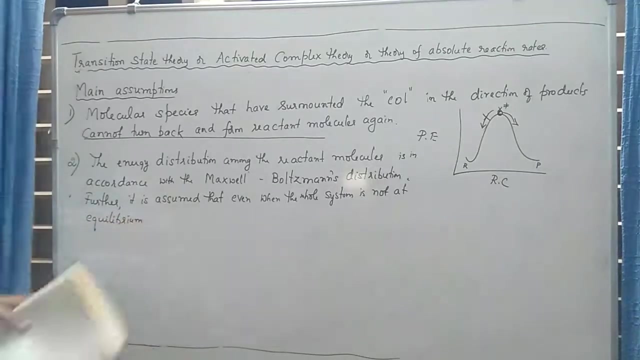 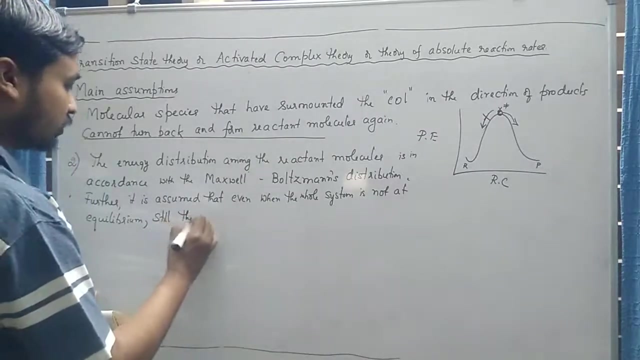 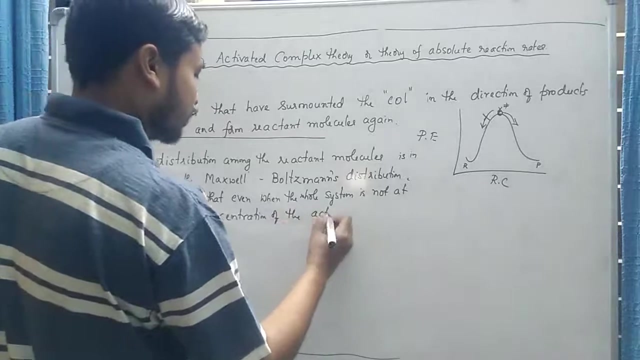 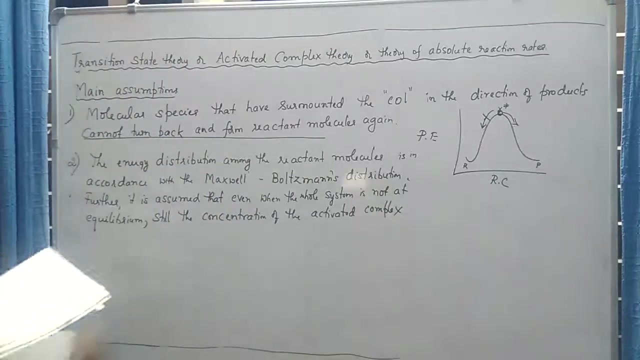 it is assumed that it is assumed that, even when the whole system, even when the entire system is not at equilibrium, when the entire system is not at equilibrium, still still the concentration of the activated complex, the concentration of the activated complex that are becoming products, that are becoming products. 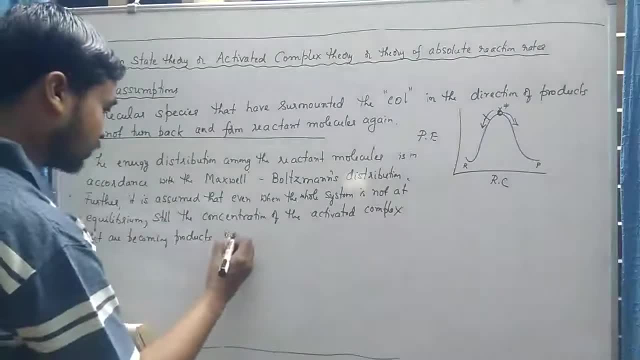 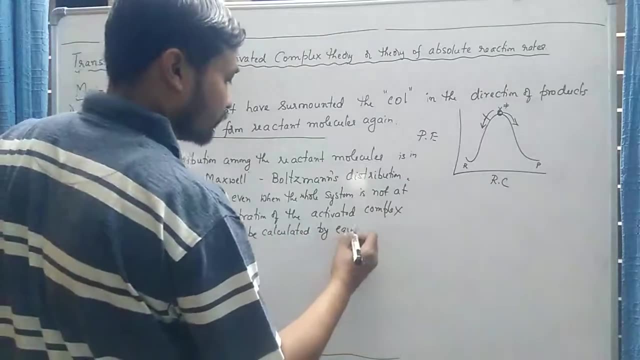 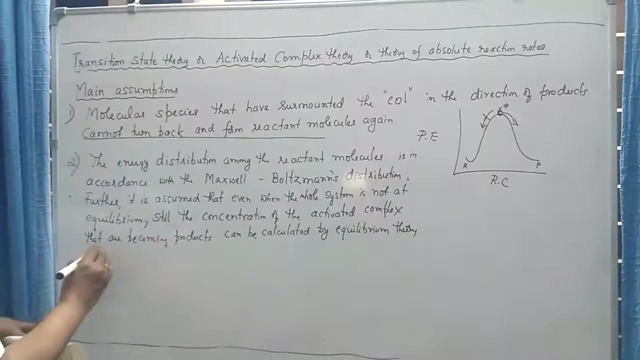 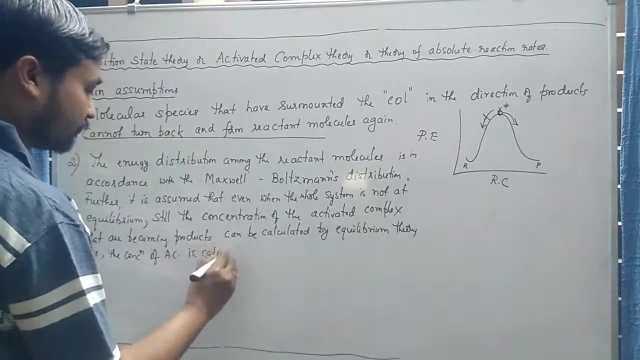 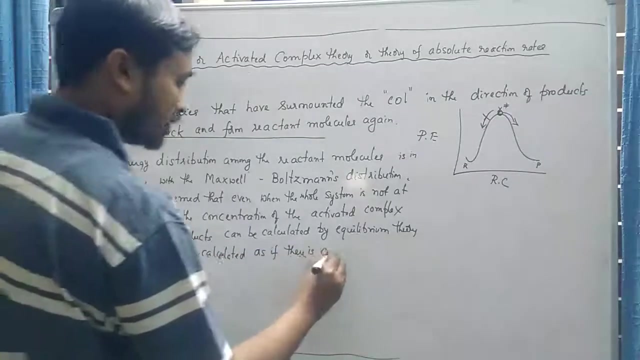 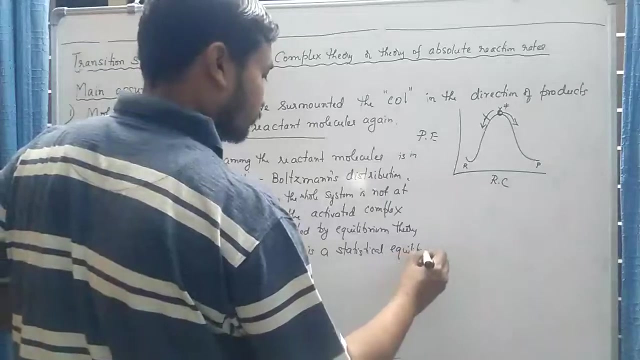 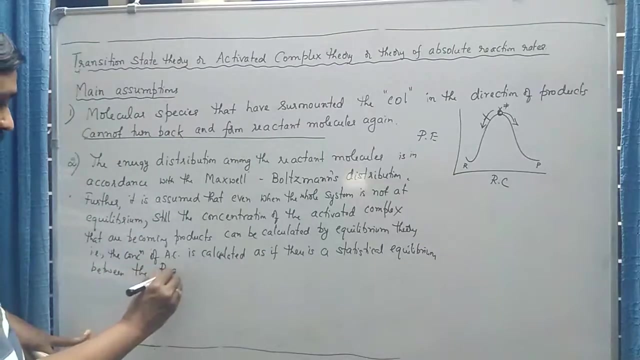 okay, is calculated or can be calculated. calculated by equilibrium theory, that is, as the concentration of activated complex is calculated, as if there is a statistical equilibrium between the reactants and the activated complex. okay, a very lengthy assumption, but the meaning is very simple. okay, so you have a lot large number of reactant molecules in the reaction mixture. okay, 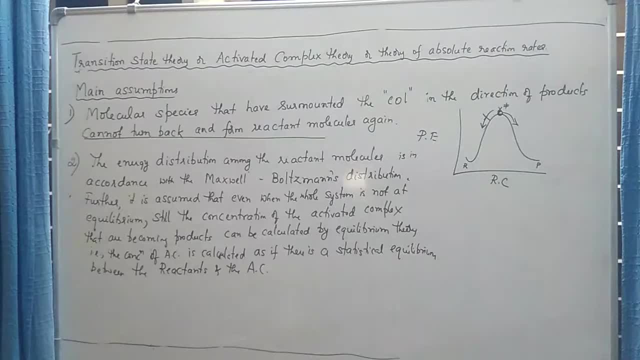 you don't carry out a reaction with one molecule of a and one molecule of b, okay. so whenever you are carrying a reaction, you mix a large amount of reactants, of the order of 10 to the power 20 molecules or 10 to the power 23 molecules- okay, are greater than that. so when you have a large 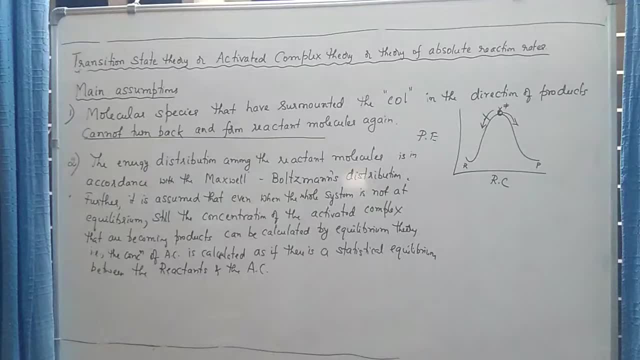 number of reactant molecules. okay, you know that the energy of each reactant molecule will not be the same. okay, the energy is distributed among the reactant molecules in different way, and how that energy is distributed is answered by the second postulate. so, according to the second postulate of 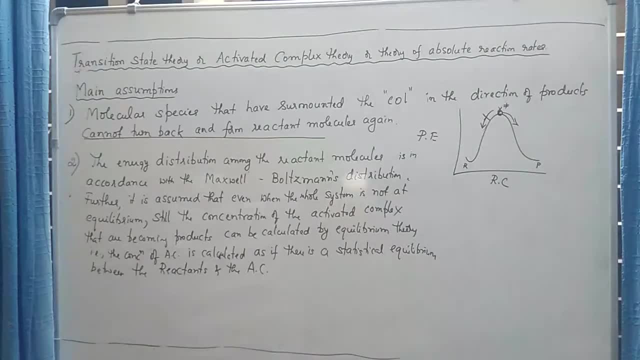 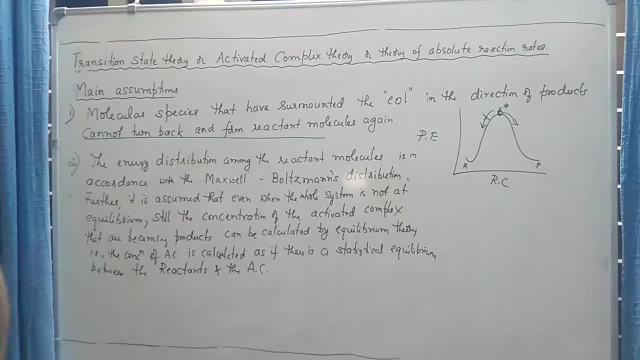 Bose-Einstein distribution. So here they have assumed that the energy of the reactant molecules is distributed in accordance with Maxwell-Boltzmann distribution. Further, this is very important. okay, I already told you there is no equilibrium between the reactant and the activated complex. 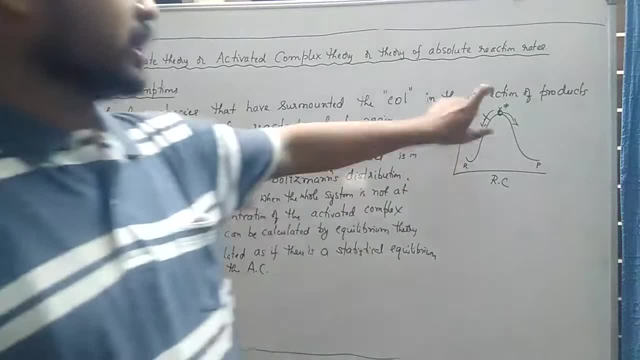 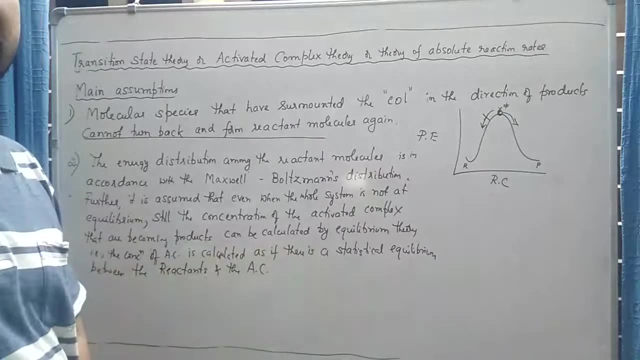 but still, in order to calculate the concentration of the activated complex, we use the equilibrium theory to calculate the concentration of the activated complex. So, though there is no equilibrium between the reactant and the activated complex, while calculating the concentration of the activated complex, it is assumed that there is some sort of equilibrium, which in fact does not. 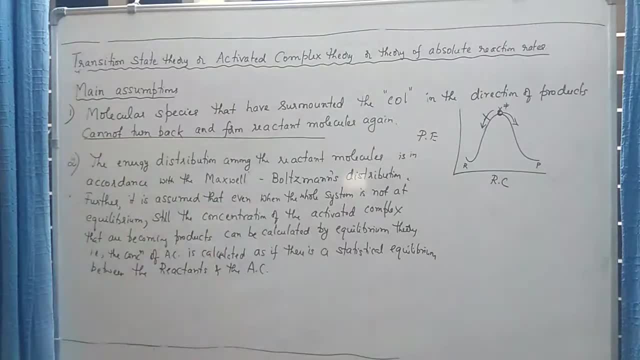 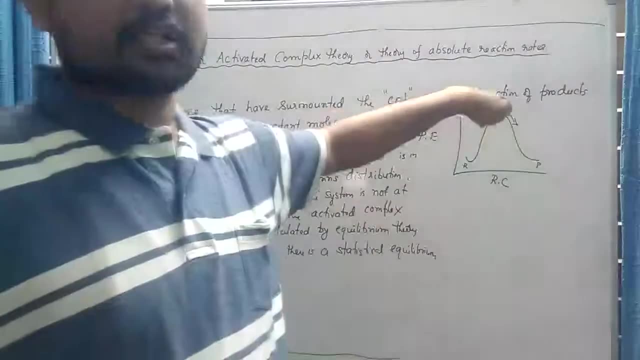 exist, but still we are using the equilibrium theory to find out the concentration of activated complex that is formed, that which is ready to form the product. Why? Because greater the concentration of the activated complex, greater is the chance of the formation of the product, which, in turn, 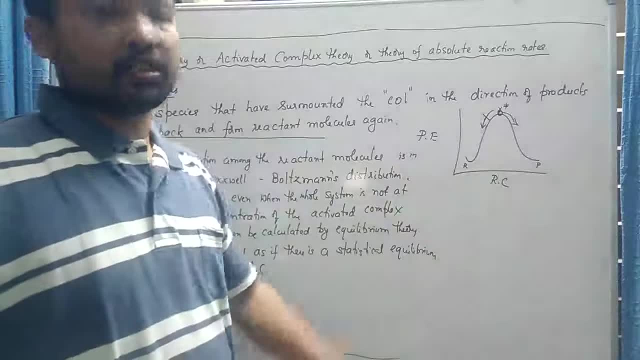 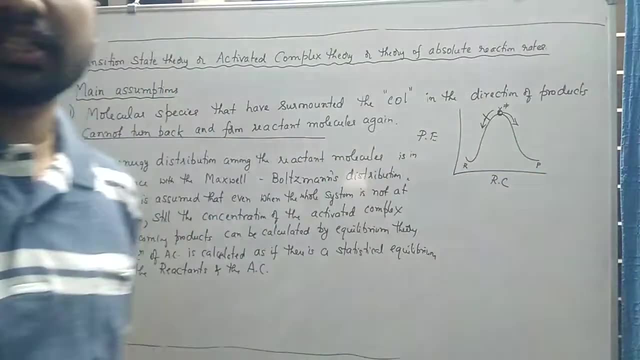 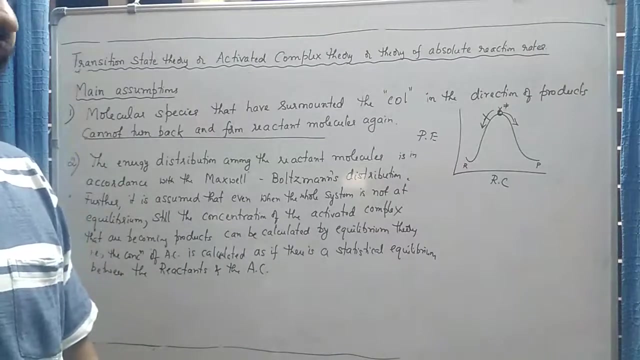 would result in the increase in the rate of the reaction. so greater the concentration of the activated complex means greater would be the chance of formation of product, and which means greater should be the rate of the reaction. So the concentration, determination of the concentration of activated complex is a very important exercise in 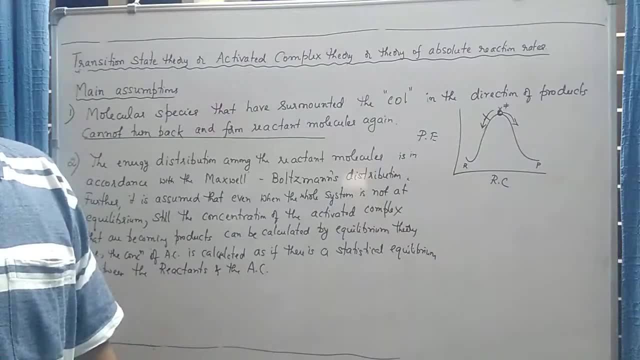 transition state theory. So how to calculate the concentration of activated complex is very important, and that is given by the second postulate, that that is, even though there is no equilibrium between the reacted molecule and the activated complex, as per the first postulate, but yet, in order to calculate the concentration of 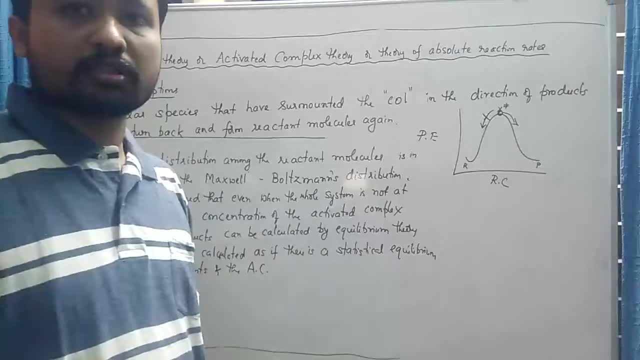 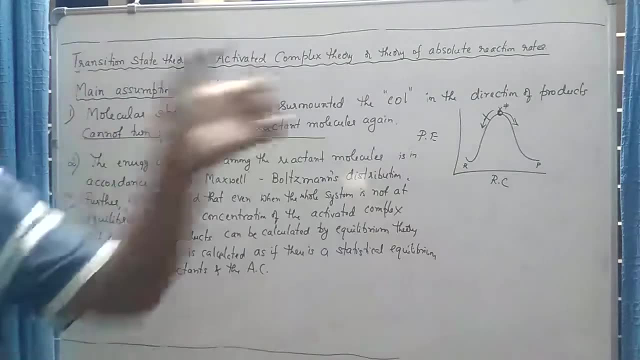 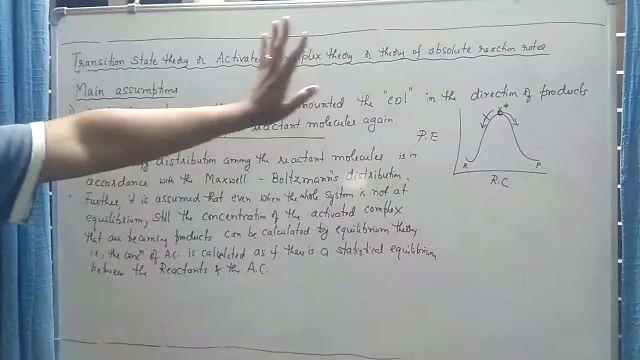 activated complex, it is assumed that there is some sort of equilibrium which actually does not exist. so we consider that equilibrium only for calculating the activated complex concentration and for no other else and for all other discussion it is assumed that there is no equilibrium between reactant and the activated complex. so this is the second postulate of activated complex theory. 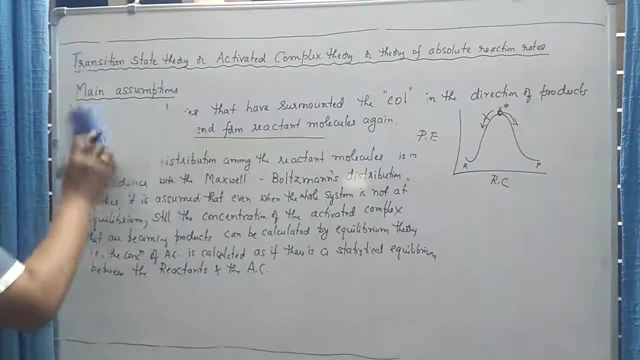 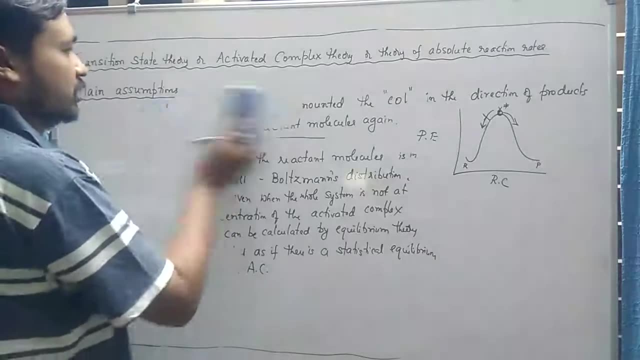 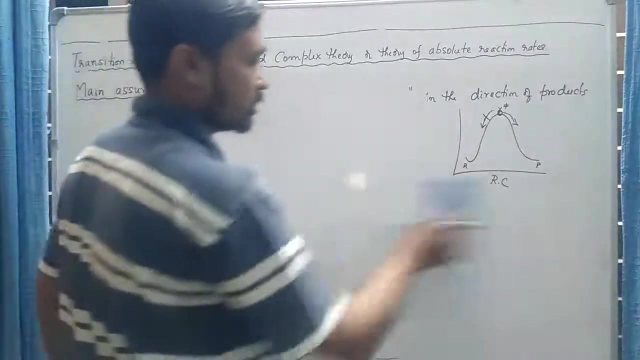 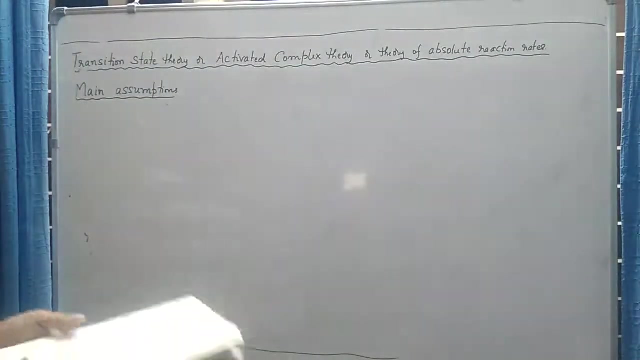 the third postulate, okay, which i will only state here. we will understand the meaning or the significance of the mean, the postulate, in the next class, when we will go into the mathematical details of this theory. okay, the third assumption of this theory is: it is possible. 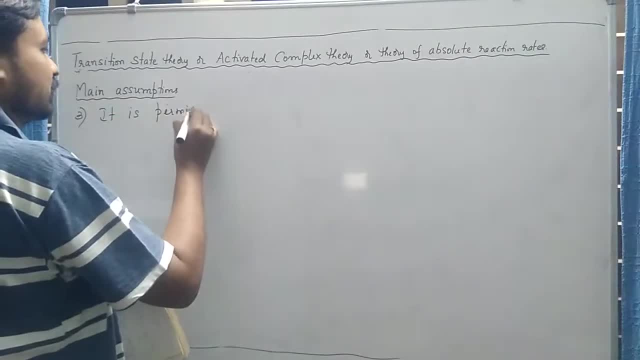 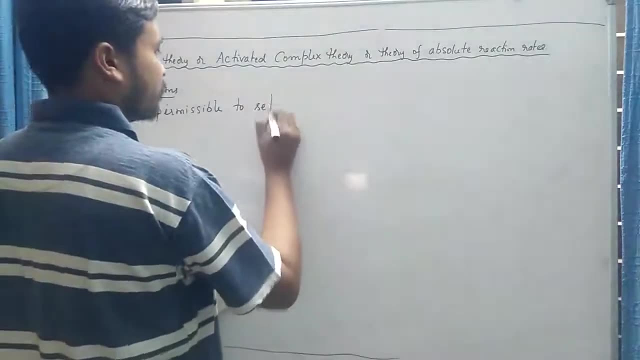 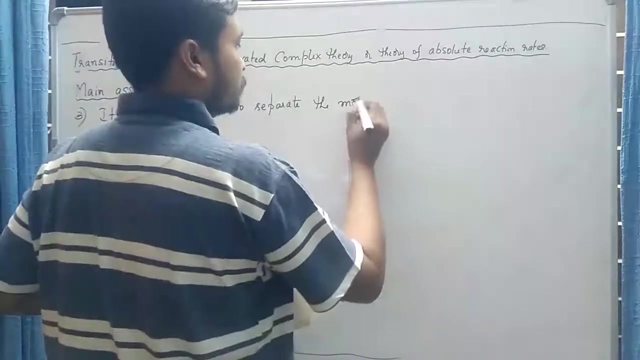 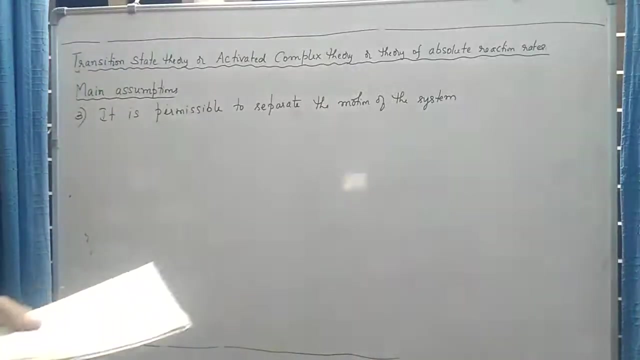 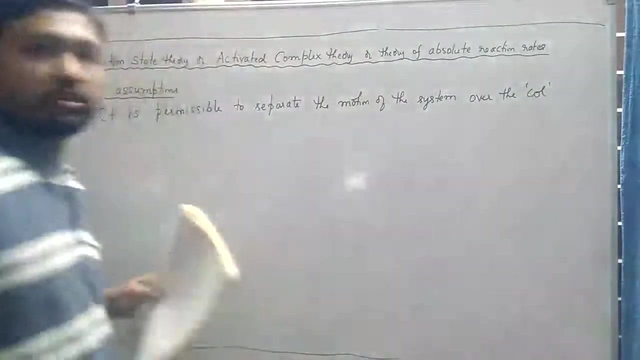 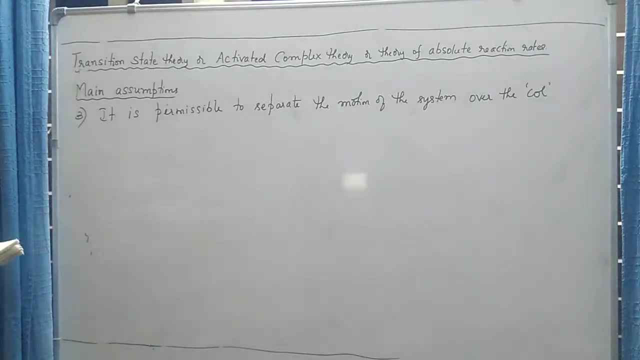 or it is permissible- okay, it is possible- or it is allowed to separate, to separate the motion of the system, the motion of the system, over the call, what is called? okay, that i already told you the barrier of the potentiality diagram. so it is permissible to separate the motion of the system. when i say system, it is actually 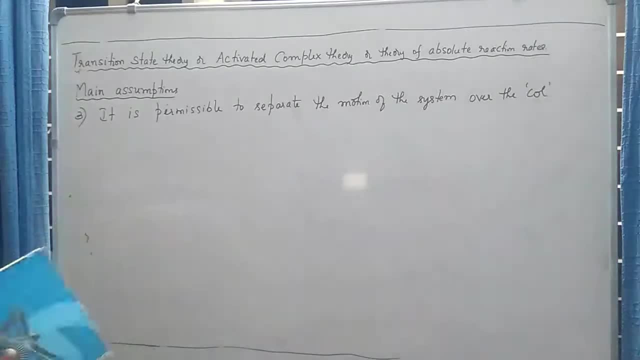 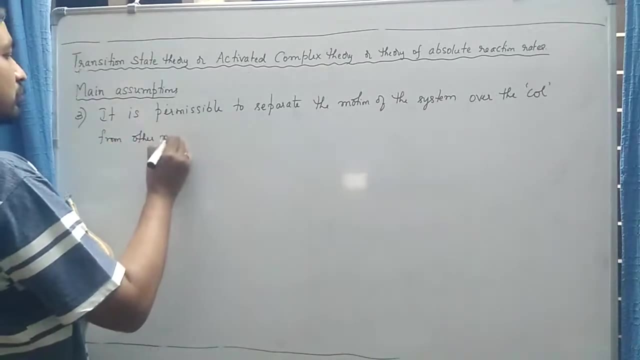 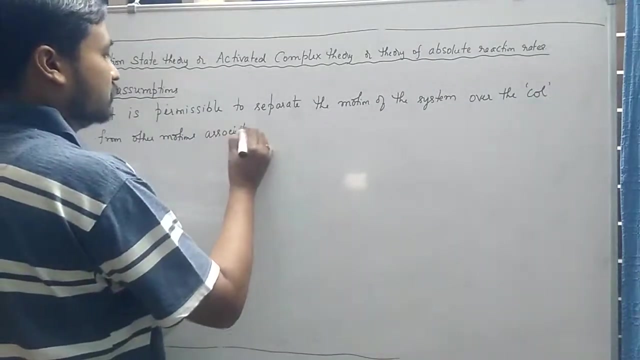 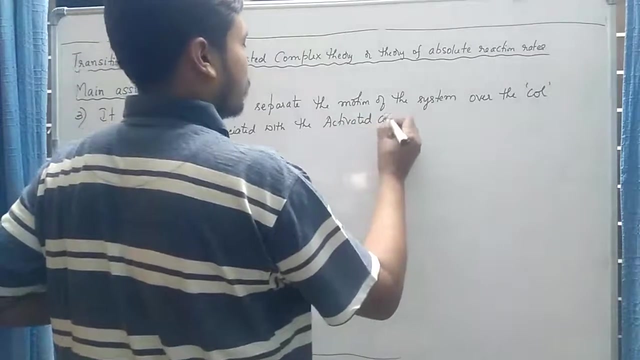 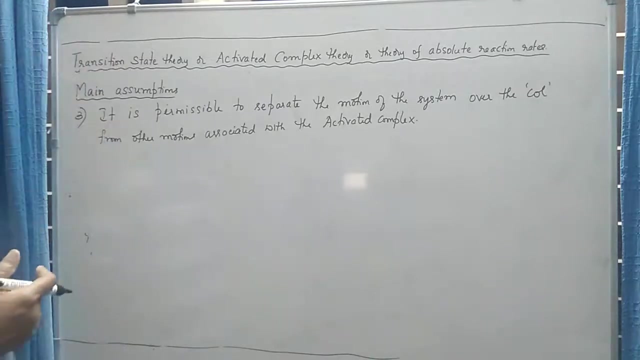 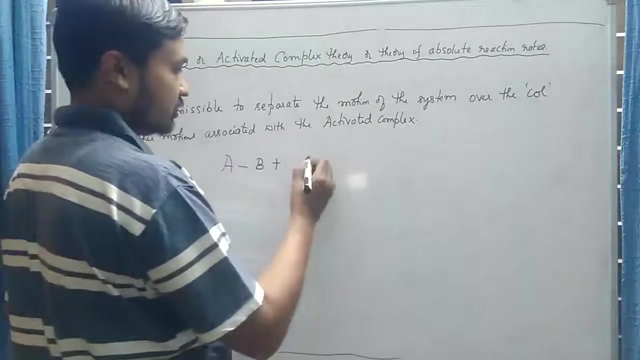 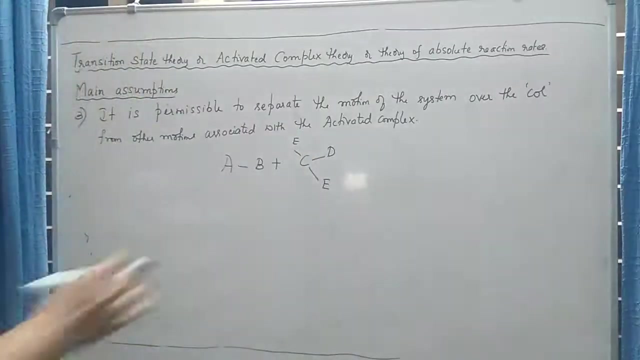 the activated complex. okay, motion of the system over the call from other motions, from other motions associated with the activated complex. okay, what is the exact meaning of this i will explain in the next class. here i will explain briefly. say, for example, this is the reaction: a b plus c, d. okay, i will take some complex structures: okay, a b plus c, d, e. okay, giving product. 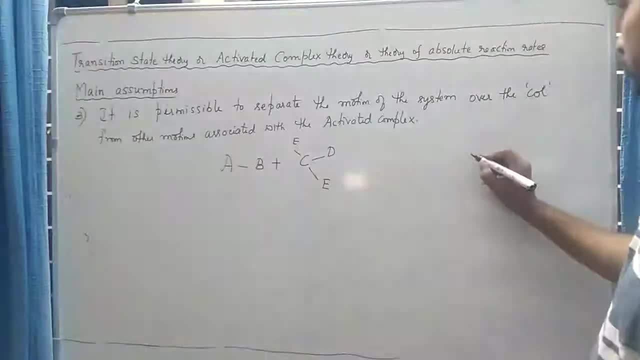 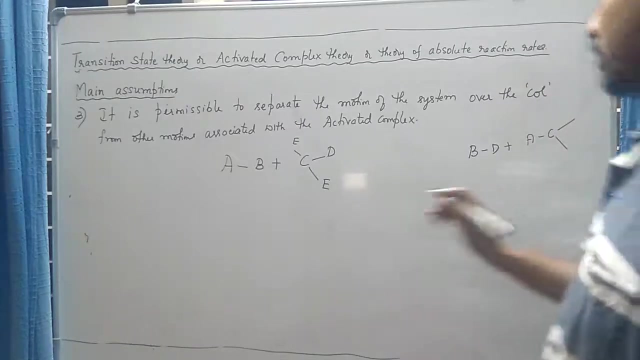 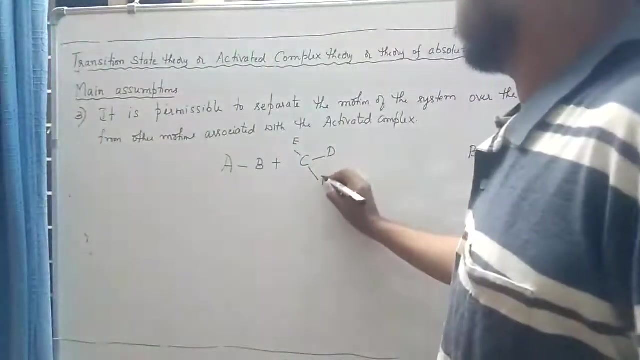 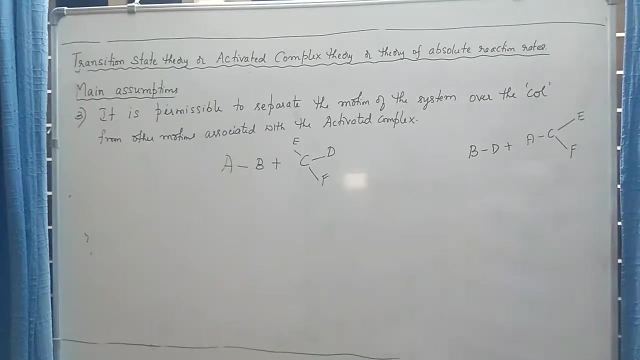 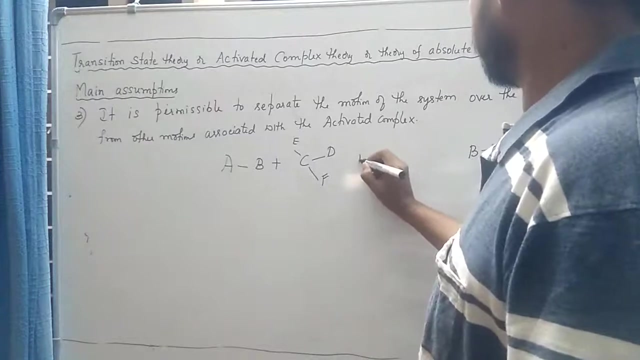 so the final product is b, d less a, c, c, f, c, c, f, a, a, e, a, e, some structure, okay, so this is the reaction. so here the activated complex has to pass through a state something like this: okay, the bond between a and b is an active complex and the activated complex needs to pass through a state something like this: 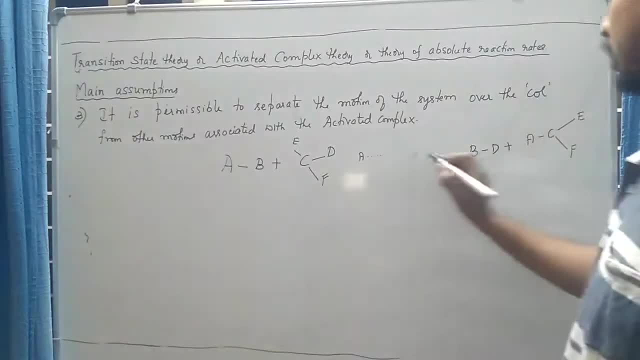 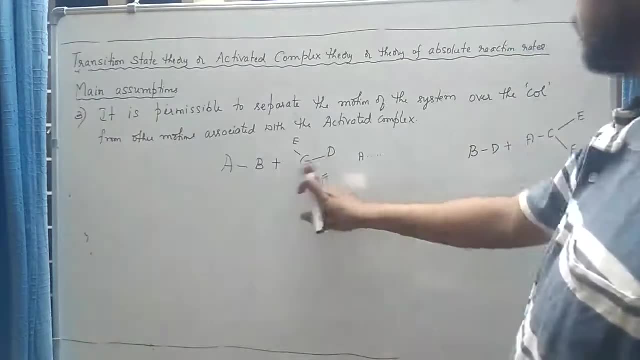 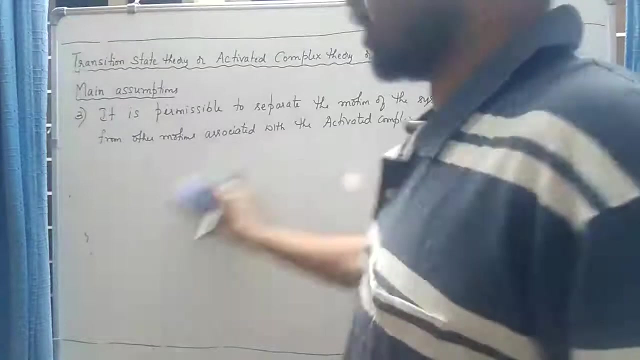 a and D. Okay, sorry, here the bond between a and B is broken. Here the bond between C and D should be broken, and a bond. Okay, I will make it to say This is very complicated. This will lead to lot of confusion. I will give you a very simple example. Okay, so a. 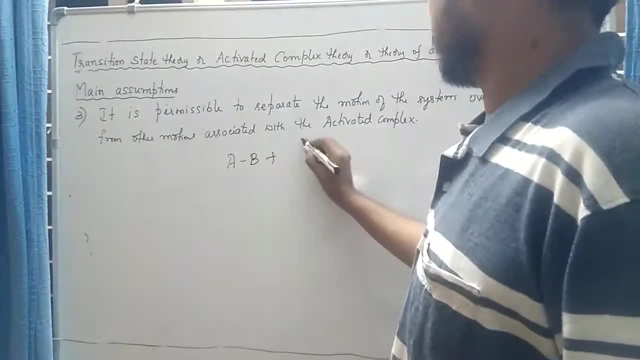 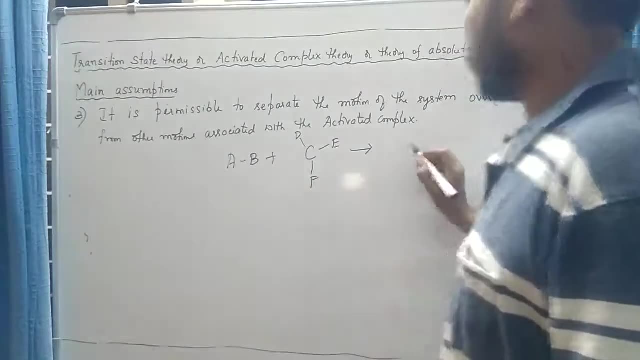 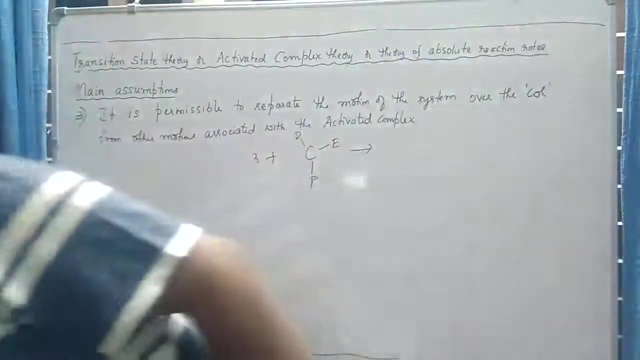 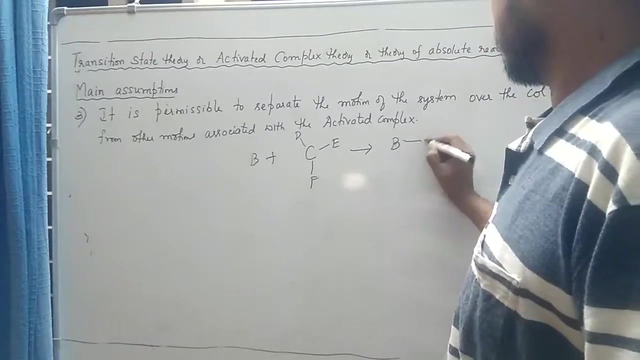 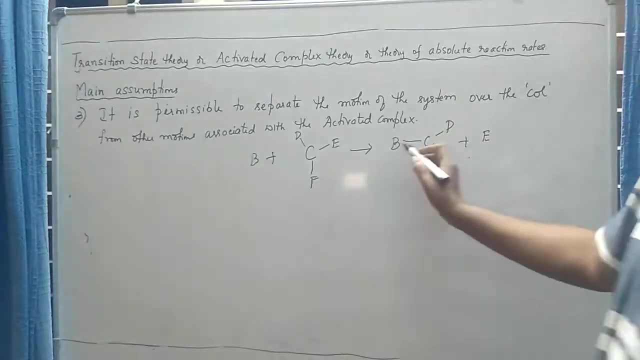 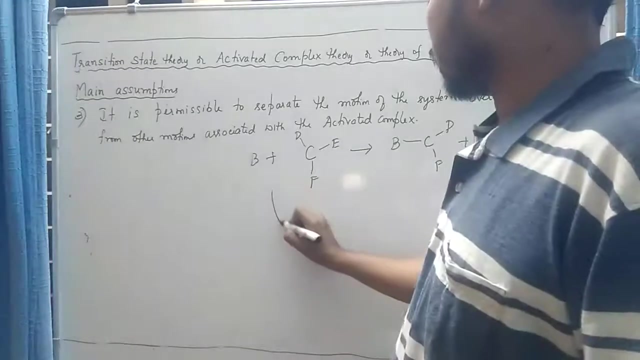 B plus C, B, E, F, Giving okay, B okay, giving B, C, D, F, Less E, Okay. so here the bond between B and C is formed and the bond between C and D is broken. So this reaction will pass through a state called transition state, where an activated complex of 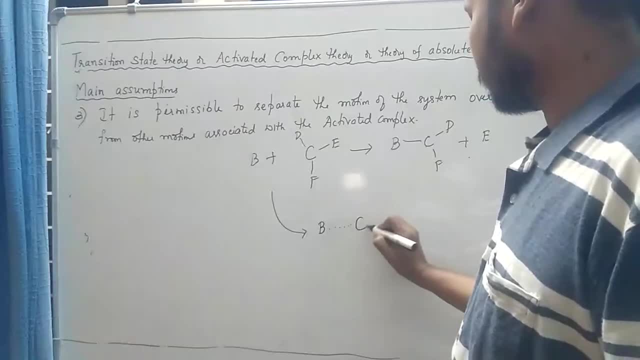 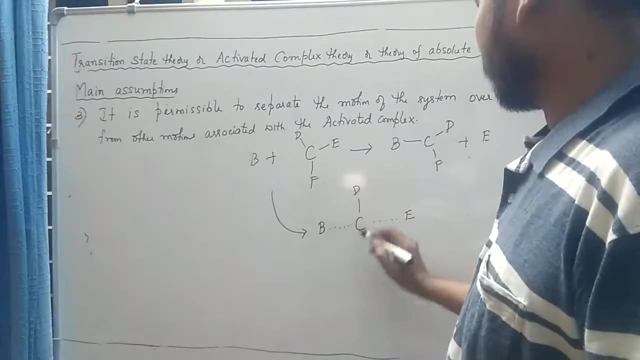 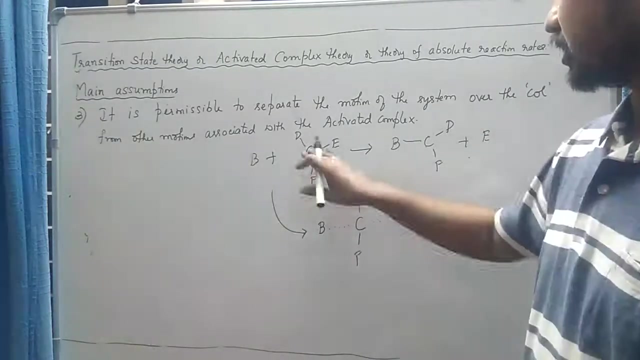 Structure something like this: bond between B and C is partially formed and the bond between C and D is completely broken. Okay, so you have D. Yeah, okay here. C necessarily is not carbon. some element, Okay, some atom, which is not carbon, Okay. so. so the activated complex has some sort of structure where the bond between B and C 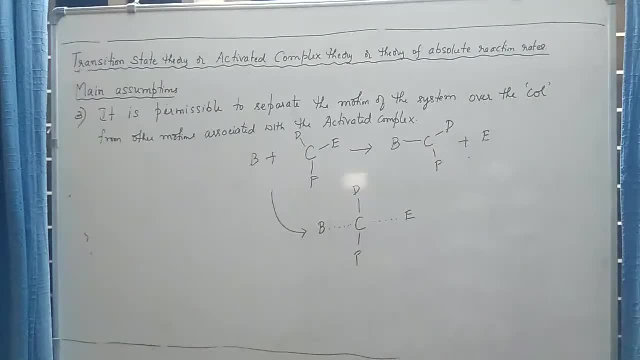 is not completely formed and the bond between C and E is not completely broken, and this finally forms the product. and For the formation of the product, the breakage of which bond is very, very important, the breakage of C- E bond is very, very important. So the vibration, 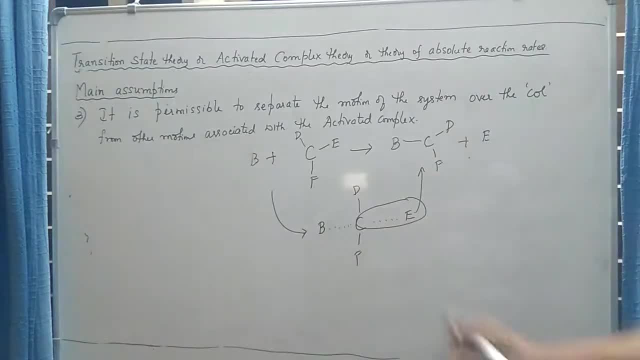 Associated with this C E bond is very, very important and, this molecule being a very complex molecule, It can perform different types of motion, It has rotational motion and it has even several vibrational degrees of freedom. Okay, There are, in fact, 3n minus 5, or 3 and minus 6 vibrational degrees of freedom, depending on whether the molecule is. 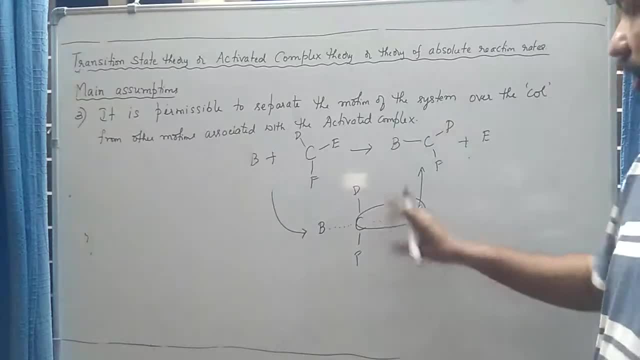 Linear molecule or non linear molecule, etc. Okay, so there are lot of vibrational degrees of freedom. Now, what this postulate is: it is possible to separate the One particular important vibrational degree of freedom, Which is the vibrational degree of freedom related to this particular bond. okay, 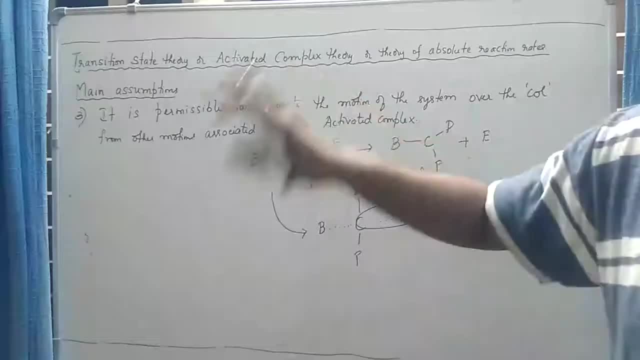 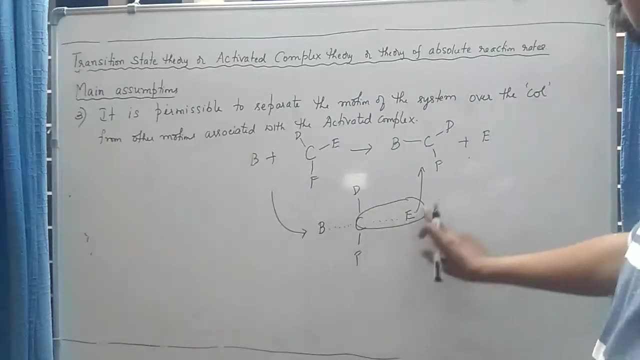 from other motions, that is, from other degrees of freedom which is associated with the activated complex. So the degree of freedom related to this particular vibration can be mathematically separated from the remaining degrees of freedom associated with this molecule. What is the meaning, exact meaning of this? we will discuss in greater detail when we go into the deeper understanding. 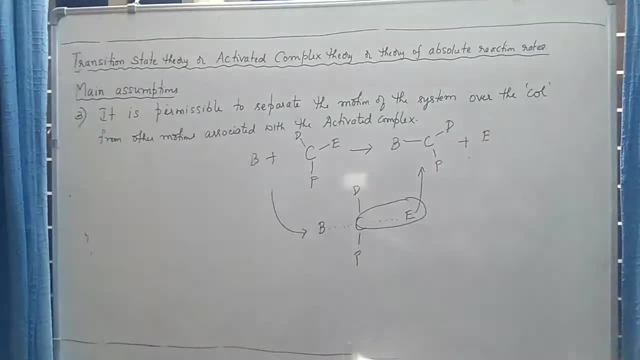 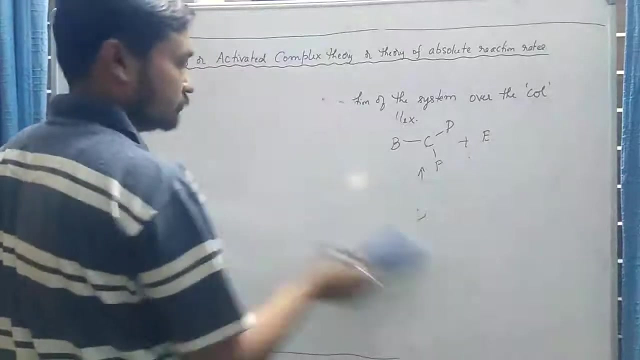 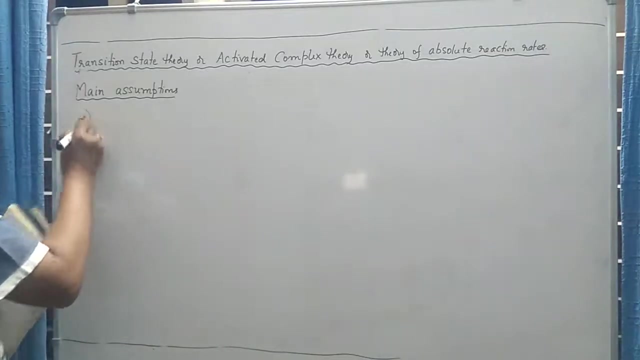 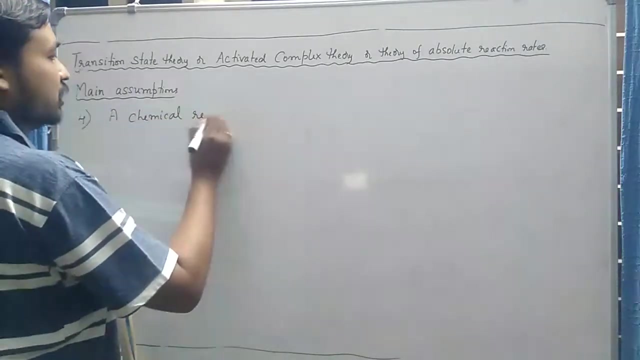 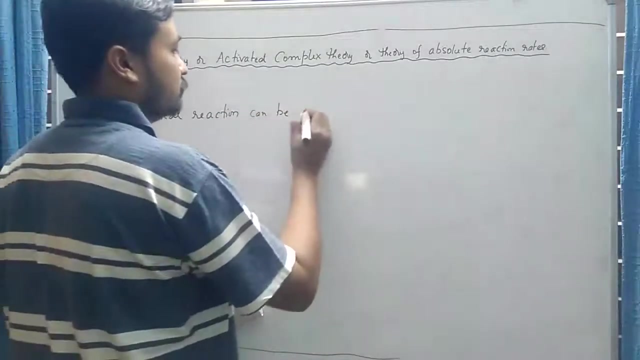 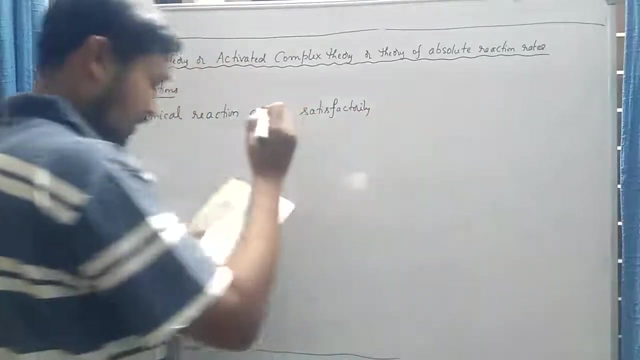 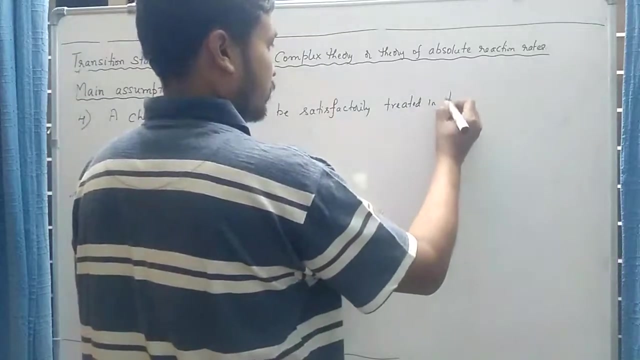 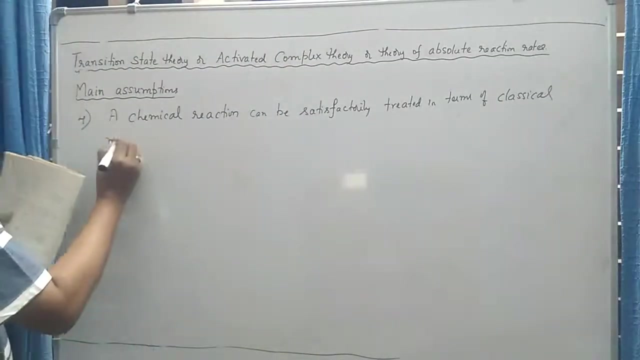 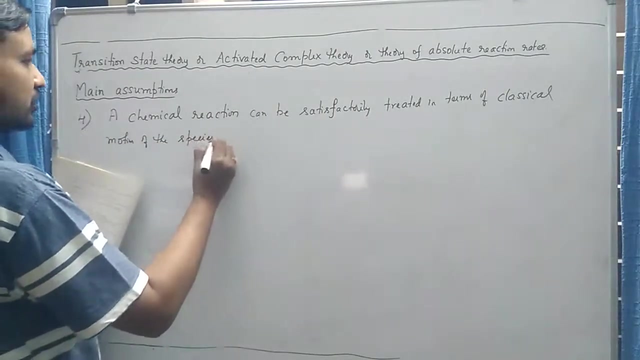 of transition state theory. So just remember what is the postulate or assumption. The fourth assumption of transition state theory is: the fourth assumption is a chemical reaction can be satisfactorily explained or treated in terms of classical motion of the Height, The motion of brutally. 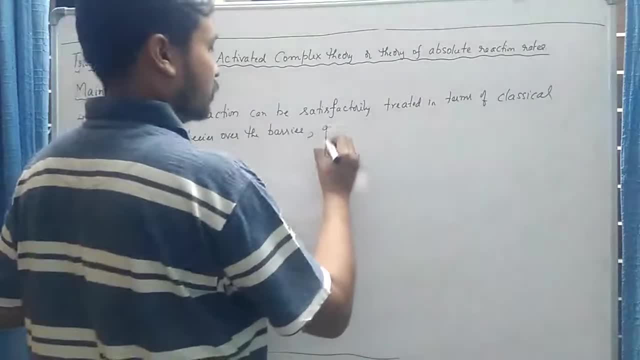 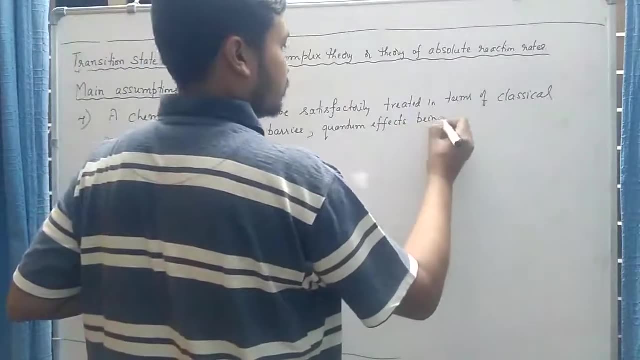 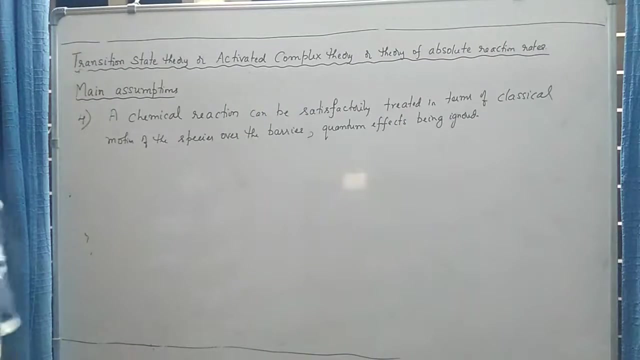 a matter of massive property in mass, of this matter for the various okay, it is in fact the quantum mechanics which gives correct result than compared to classical mechanics. but here they postulate that, or they assume that the chemical reaction between the two molecules, okay, can be satisfactorily. 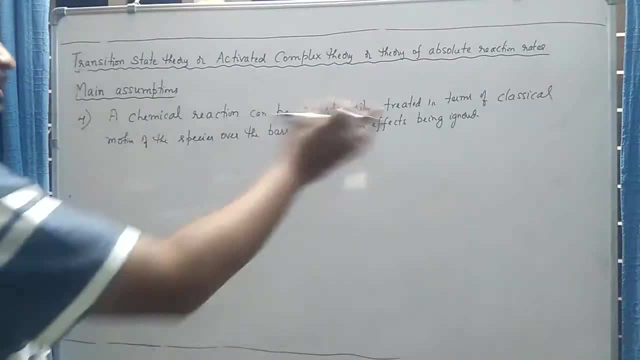 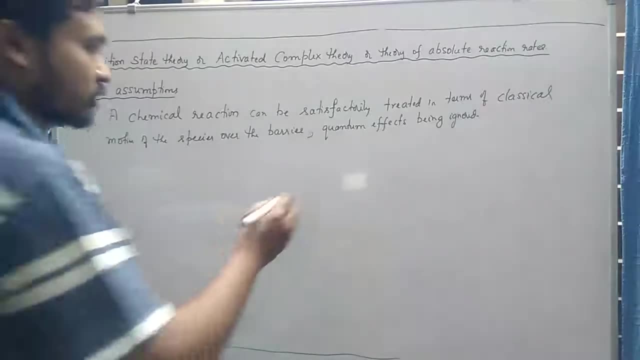 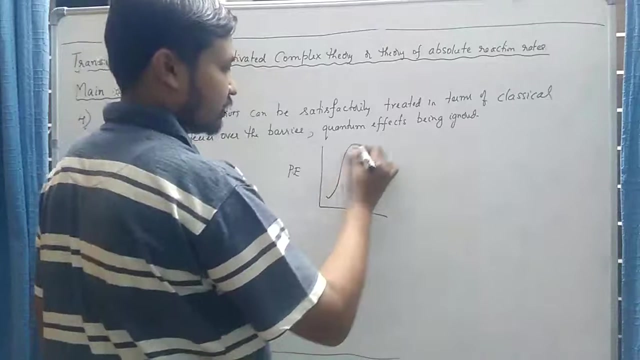 treated or explained in terms of classical motion of the species over the barrier. okay, quantum effects being ignored. what is the meaning of this? let us try to understand so again, I will draw the potential energy diagram versus reaction coordinate. okay, this is how a potential energy diagram generally looks. 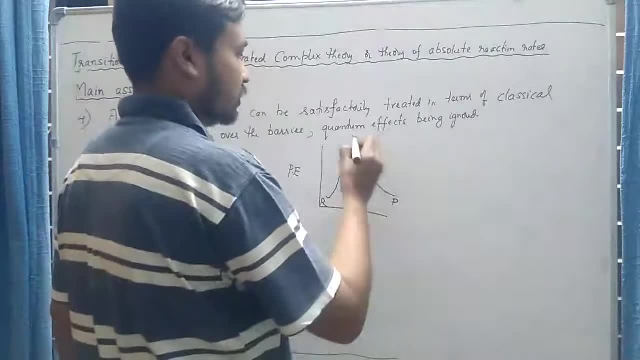 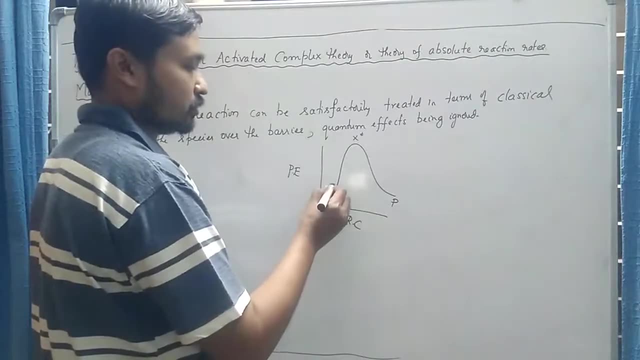 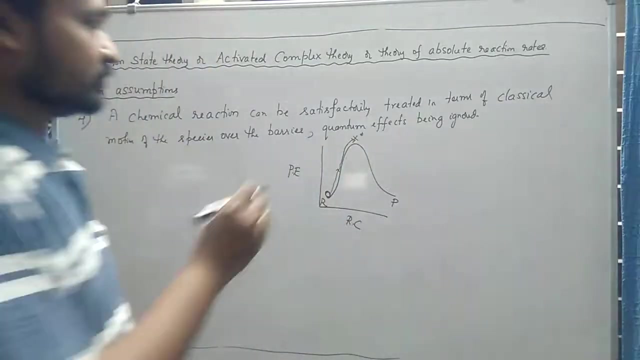 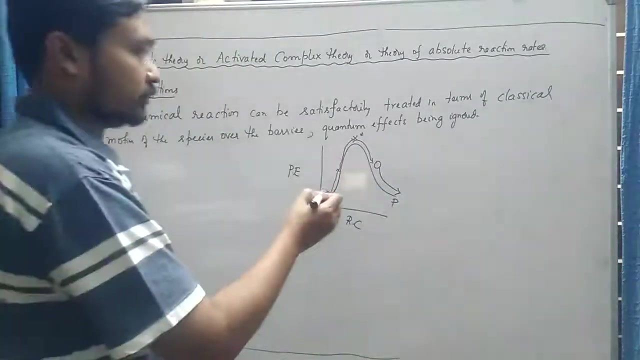 so this is the reactant, this is the product and this is the activated complex. so a reactant molecule, okay, it slowly claims this hill. it claims this hill became. it involves an activated complex and this activated complex will roll down and form the final product. so the motion of this molecule, okay, the molecule. 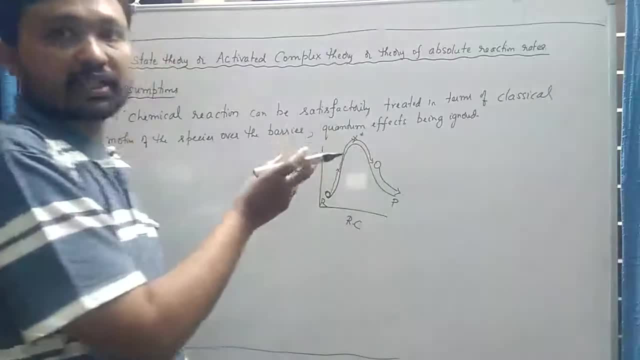 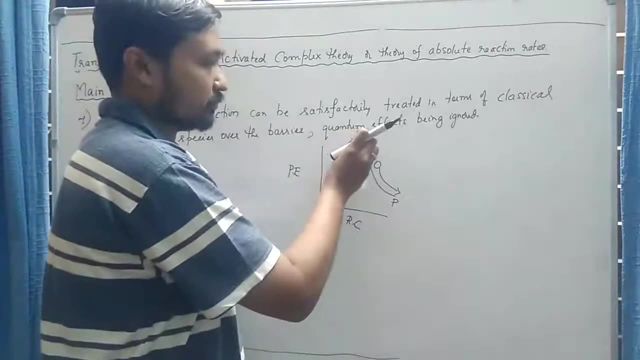 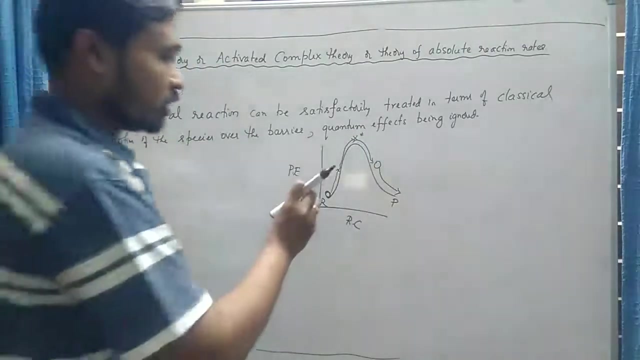 initially its reactant. when it reaches this particular stage, it has returned a transition state where this species is an activated complex, okay. further, the motion of the species along this potential of the diagram. and finally, when it reaches here state. so the motion of the species above this potential energy diagram. okay so. 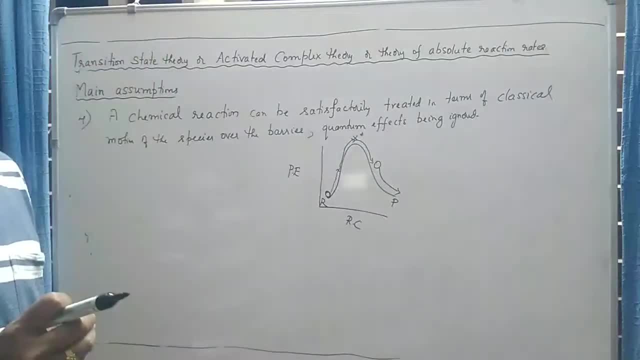 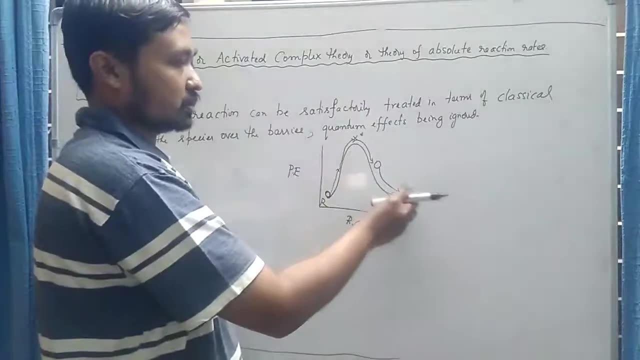 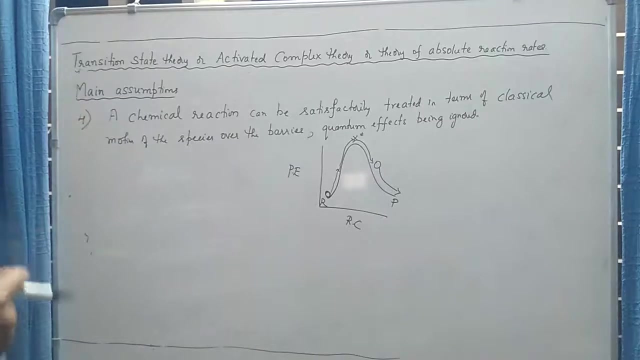 this motion is assumed to be a classical motion. it means it follows the rules of classical mechanics. strictly speaking, the motion of the molecule along this barrier should be treated by using the rules of quantum mechanics, but here they assume that, okay, we get a satisfactory result even by considering the classical 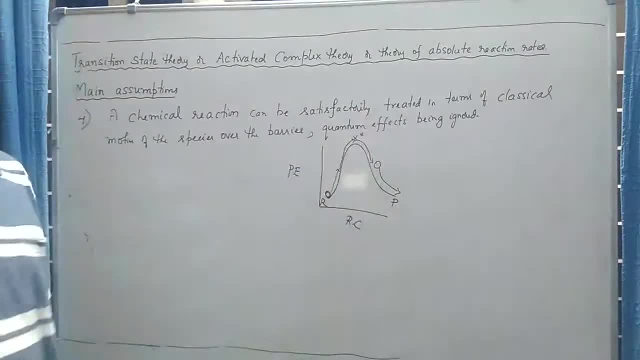 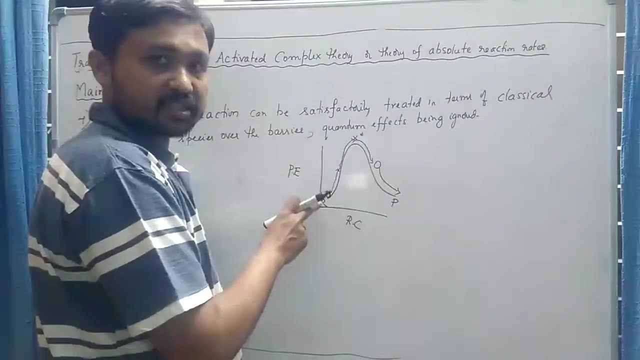 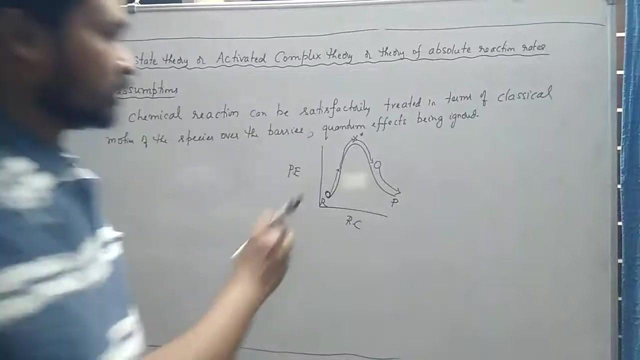 motion of the species over the barrier, ignoring quantum effects. okay, what does this quantum effects do? according to classical theory, reactants suppose the reactants has to get converted into product. it has no other way other than crossing this barrier and forming, finally forming the product. there is no. 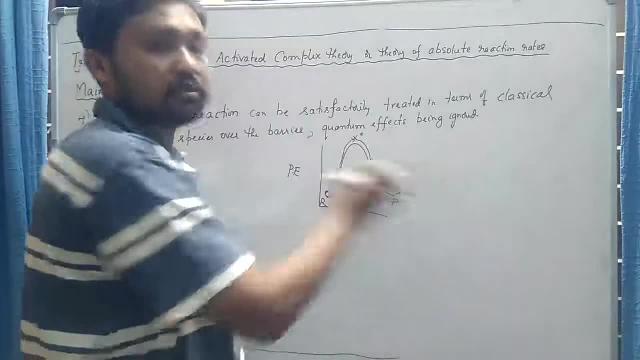 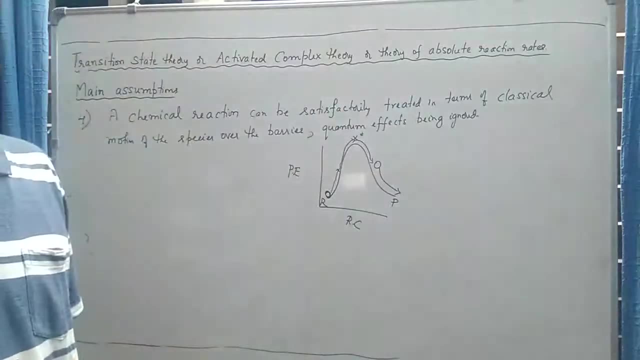 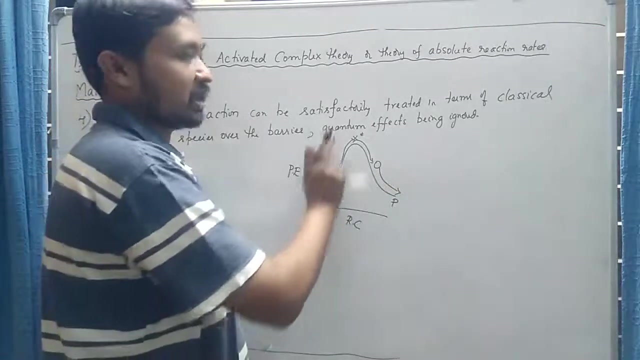 shortcut method for the reactant to form product, it has to climb this barrier, form the activated complex which rolls down to form the product. this is called what is the classical theory expects. if I want to reach from here to here, the only one way that is possible is to climb the hill. 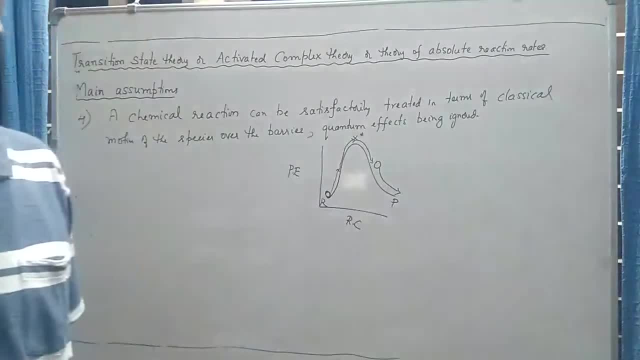 pass to the other side. that is the classical idea, whereas according to quantum theory, if I apply the Schrodinger wave equation to this system and solve the Schrodinger wave equation, it gives a very important result, which is called a tunneling effect. so what does this tunneling effect do? is okay. 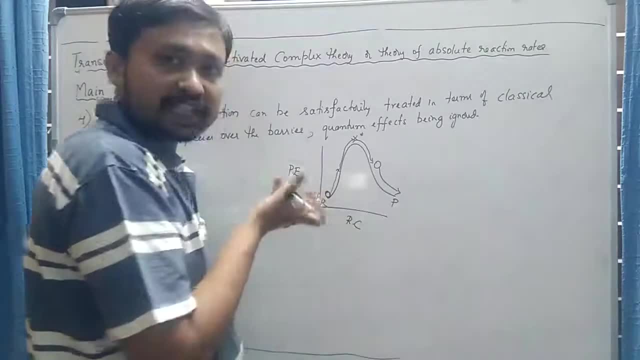 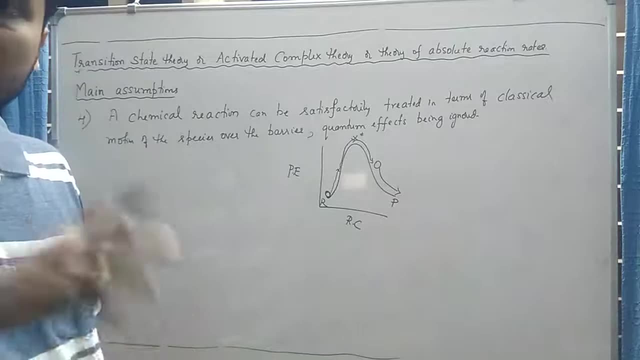 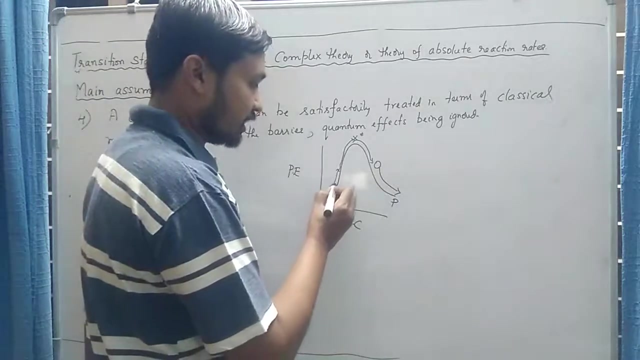 the reactant molecule, even though it has not gathered enough energy to overcome this barrier, there is a possibility or probability that the molecules, even without achieving that minimum energy, has a probability to form the product. okay, that phenomenon is called as tunneling effect. so the reactant molecule, due to pollution it has gathered. 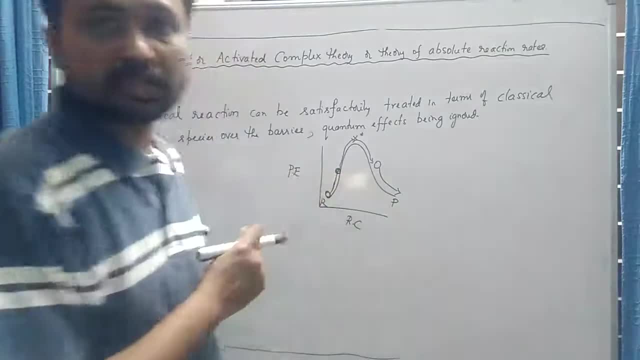 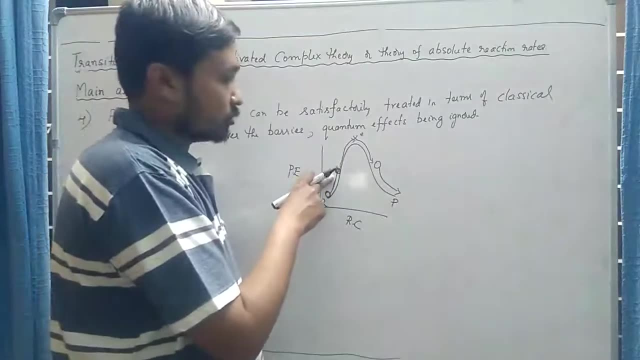 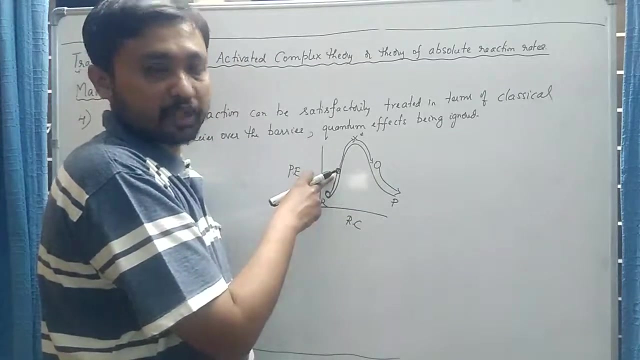 some energy and it has reached here which is not, definitely not the maximum energy. so this is not the transition state or this is not the structure of the energy of an activated complex. so according to classical theory, if the molecule has attained this, this much energy, it is no way eligible for forming the product in. 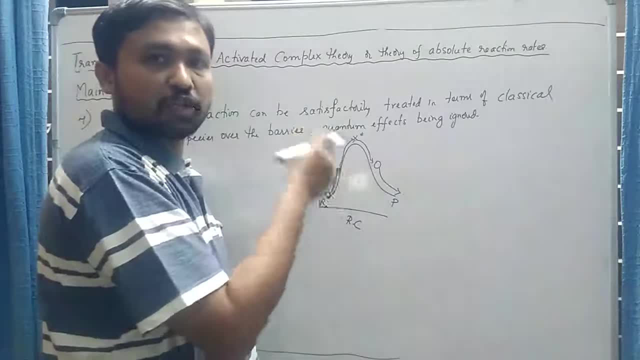 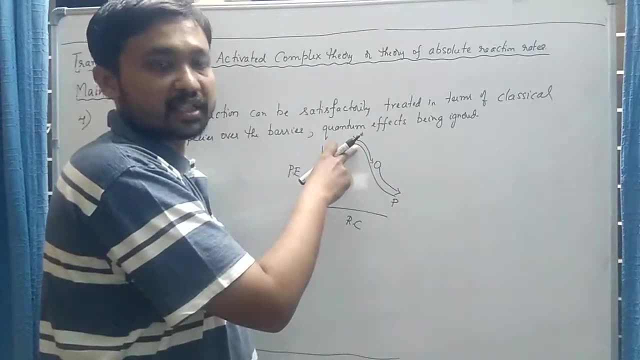 order to perform the product, the molecule has to gain more energy, more and more energy by collision. it has to reach the top of this barrier. until and unless it reaches the top of the barrier, it cannot form the product. this is the classical picture. but according to quantum theory, if the molecule has 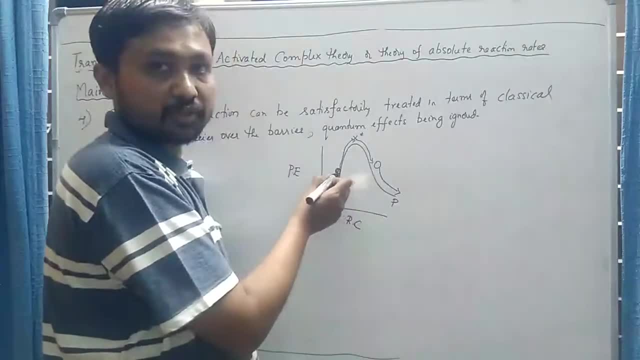 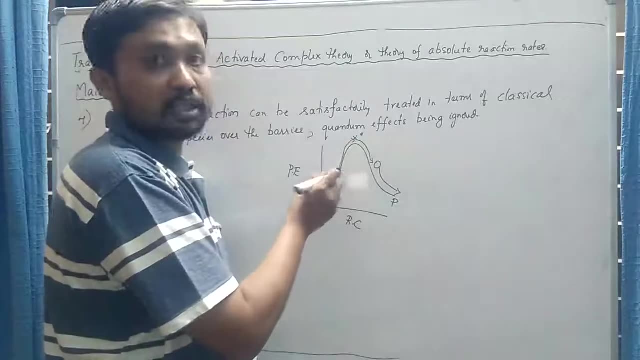 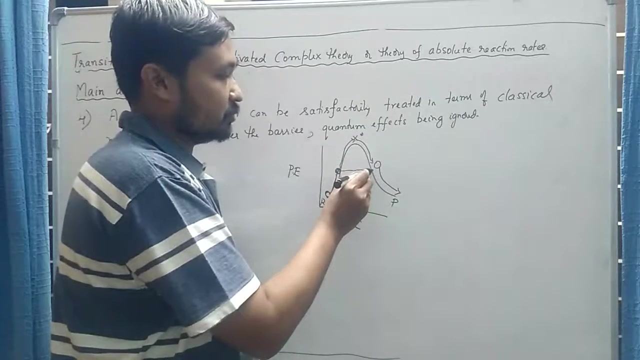 attained energy corresponding to here what I've shown here. there is a probability that even this molecule, without crossing the barrier, can form the product. so there is some sort of tunneling that happens within this barrier, okay, and the molecule will reaches here, which will roll to form the final product. so, without reaching this, 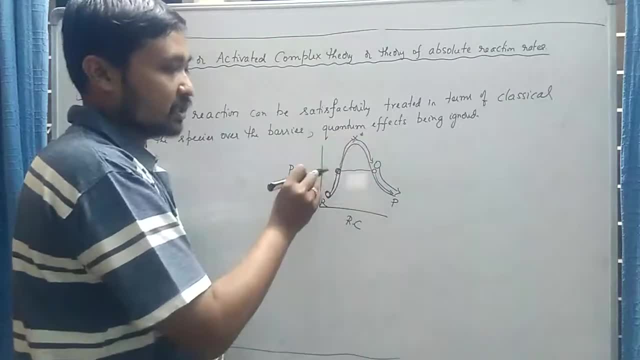 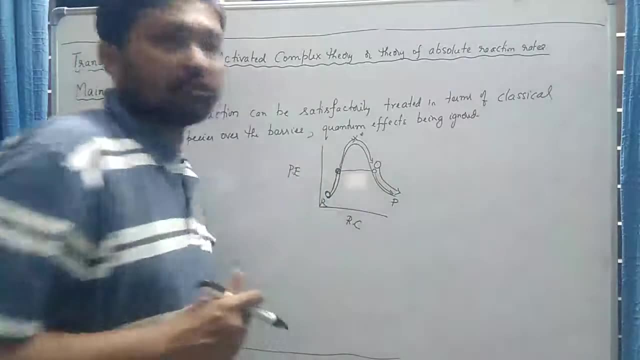 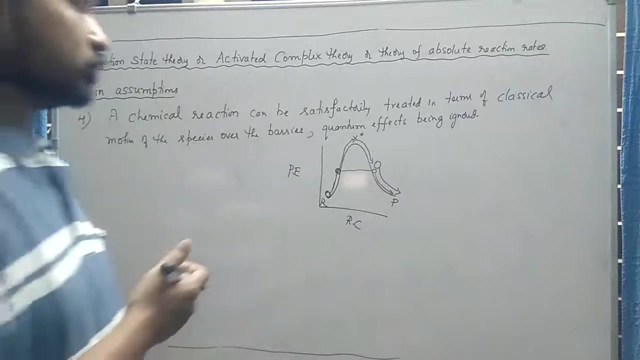 maximum energy state without formation of the activated complex. this molecule will tunnel through the barrier and form the product. so this type of results we get from quantum mechanics if we apply quantum mechanics. so quantum mechanics allows the possibility of tunneling, but here they are assuming that such 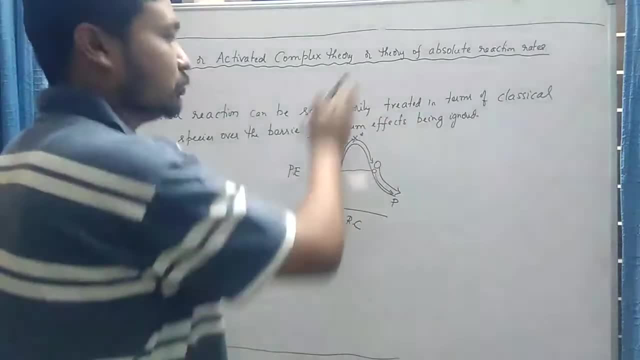 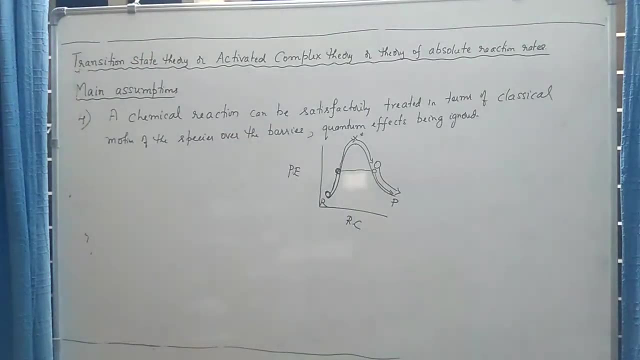 complicated theories need not be applied. even the classical motion of the particle through the barrier is suffice or sufficient to get desirable or appreciable result. okay, so this is the meaning of the the fourth assumption. the fifth assumption is that the particle is not moving through the barrier and the 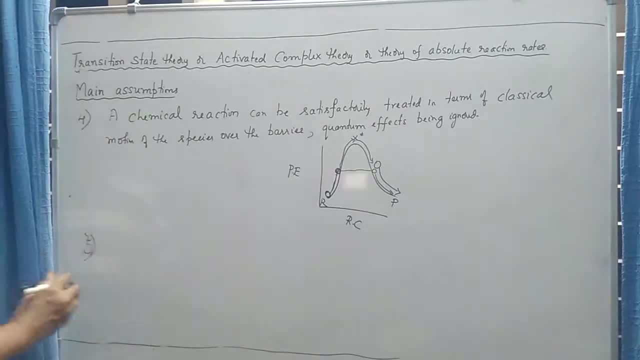 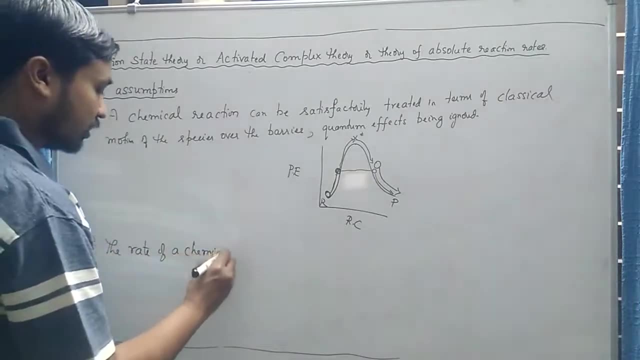 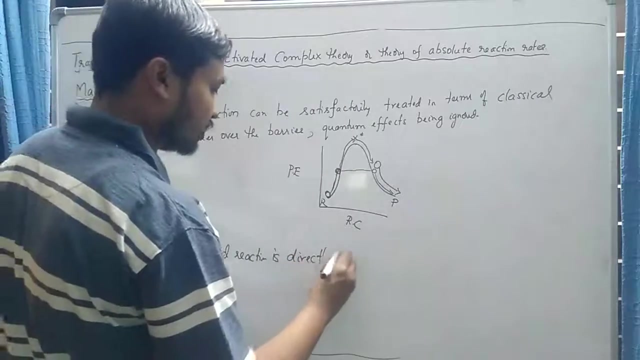 MUELLERобод, czyli yes, it is situated nothing. so now we need to further analyze the point. we are applying quantum mechanics. our Arctic equation works like this. so if we have one chemical and oneicle, we want to call it like this and by doing the 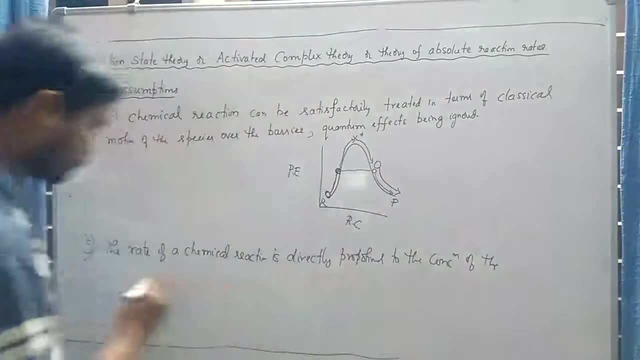 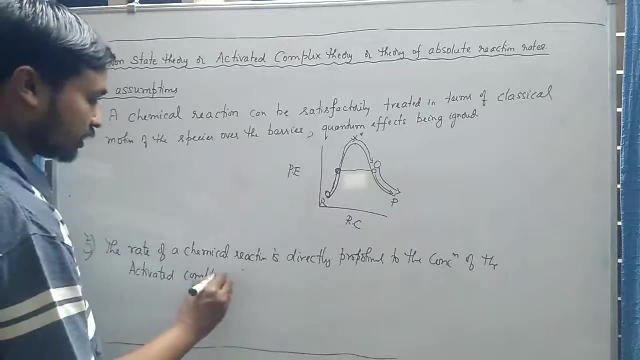 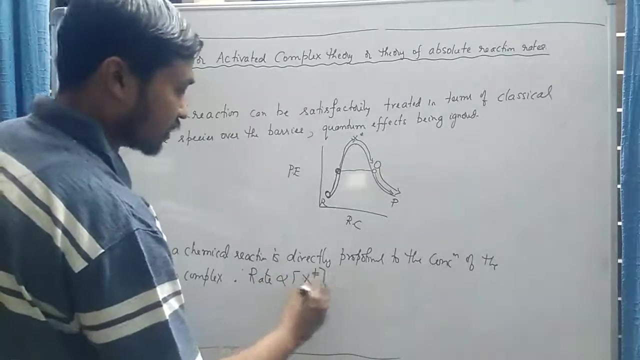 to sum the relation of the reaction from the particle point to the material. this would be related to the very first assumption, or the couplet or any other activated complex. okay. so the rate is directly proportional to concentration of the activated complex that is formed, okay, which is ready to form the final product. this i have explained.